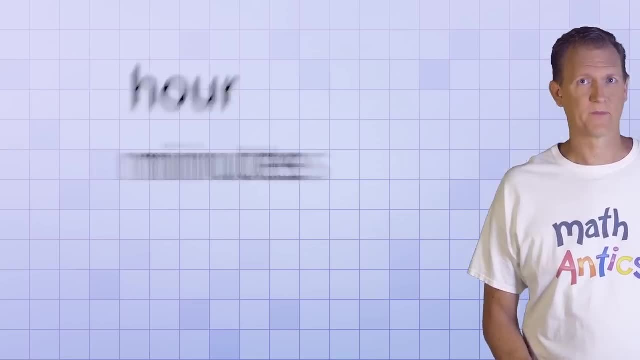 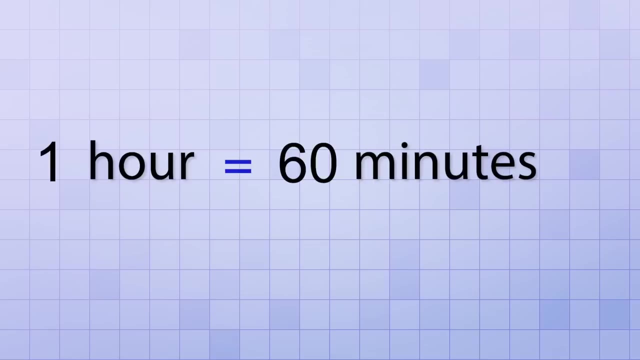 So we divide hours up into even smaller units, called minutes. Specifically, each hour is divided up into 60 minutes, So a minute is 1 60th of an hour. And to get even smaller units of time, we divide up each minute into 60 equal parts. 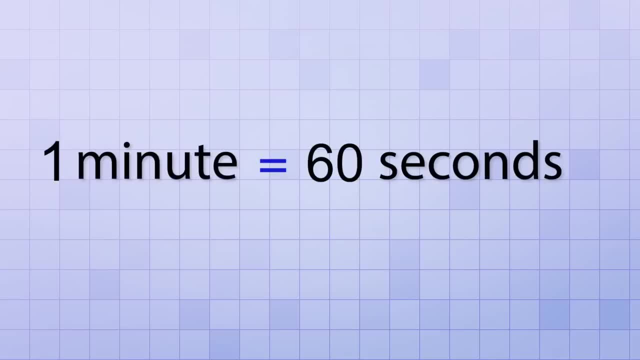 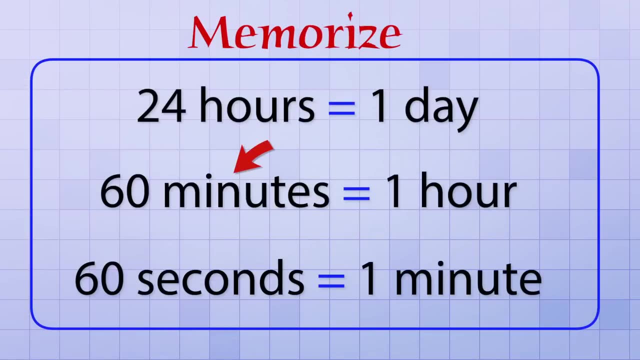 called seconds. So a second is 1 60th of a minute, Going from the smallest to the biggest. you should memorize that 60 seconds equals 1 minute, 60 minutes equals 1 hour and 24 hours equals 1 full day. 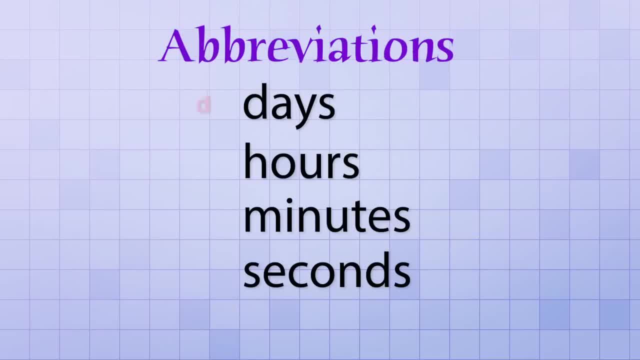 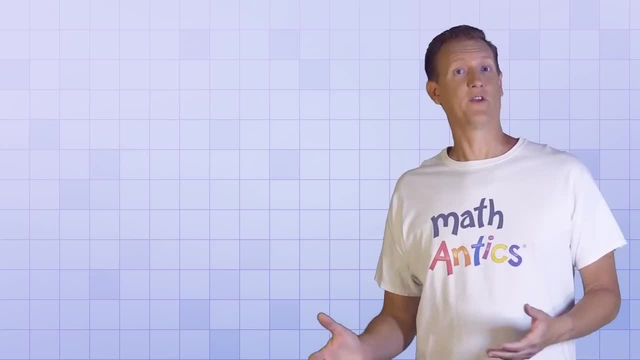 There are some common abbreviations for these units that you should know too: D for days, H for hours, min for minutes and s for seconds. One of the earliest devices for measuring time was called a sundial. It was basically a flat disk…. 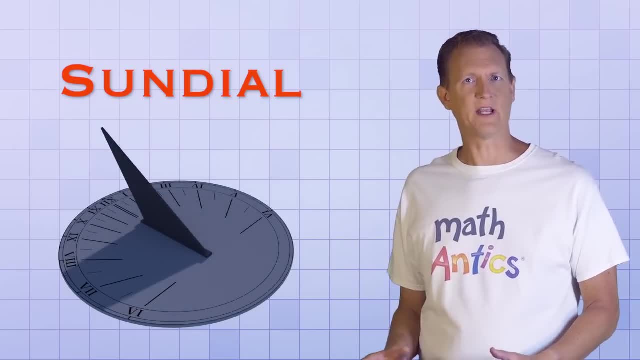 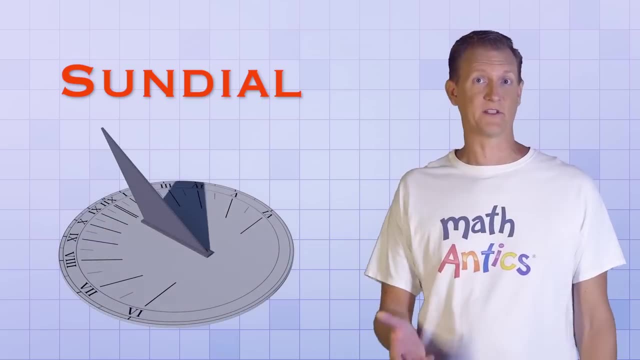 …with a triangular pointer in the middle. As the Earth rotated, the shadow of the pointer would slowly change position and point to different markings on the edge of the circle which represented different times of the day. Are you tired of the man telling you what time it is? 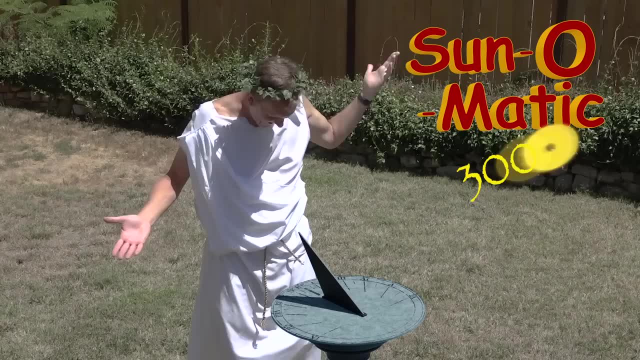 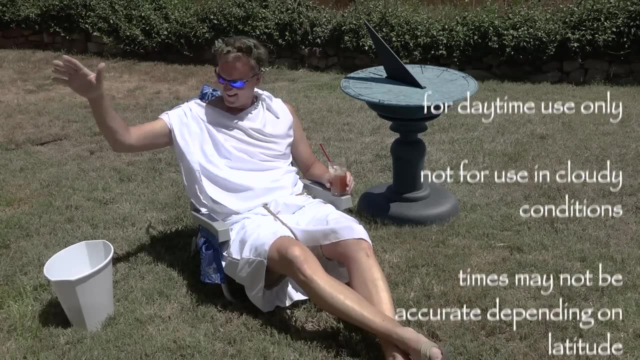 Now you can get the time directly from the source with the Sun-O-Matic 3000.. Just put it in your yard and let the sun do the rest. For daytime use only, not for use in cloudy conditions. Times may not be accurate depending on latitude. 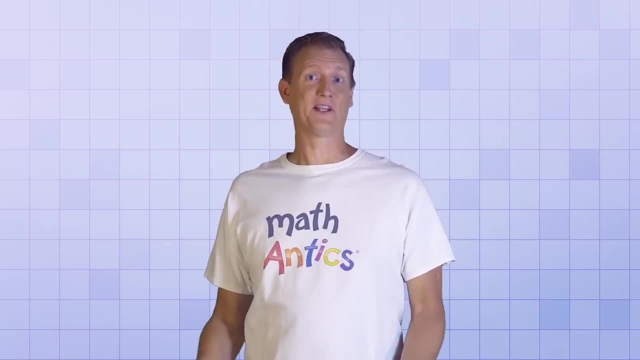 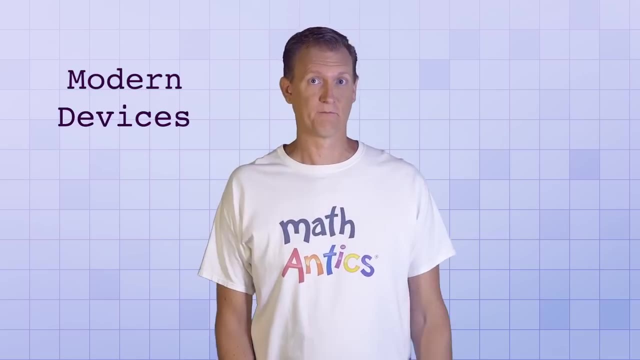 Some calibration required. The sundial was a really cool invention, but it had a lot of limitations. Fortunately, there are much better, modern devices for keeping track of time. In fact, you probably have one hanging on your wall at home or in your classroom that looks. 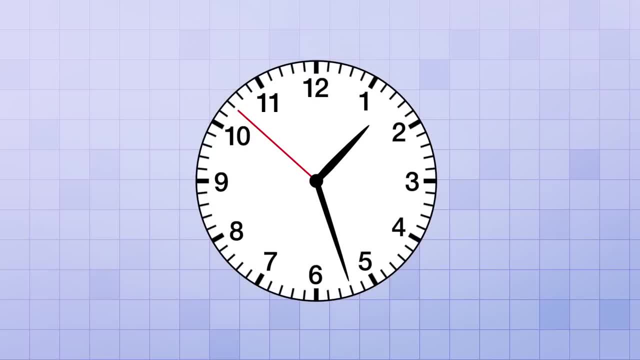 something like this. This traditional clock is designed to keep track of 3 different units of time: Seconds, minutes and hours. That's why it has 3 different pointers or hands. This thin red pointer is called the second hand because it helps us keep track of seconds. 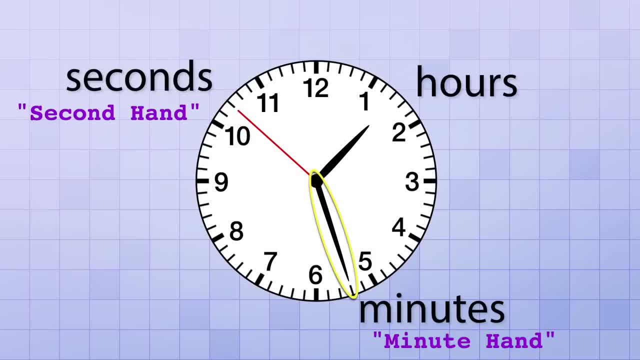 this thicker black pointer is called the minute hand because it helps us keep track of minutes, and this shorter black pointer is called the hour hand because it helps us keep track of hours. Oh, and the circle itself is often referred to as the clock face. 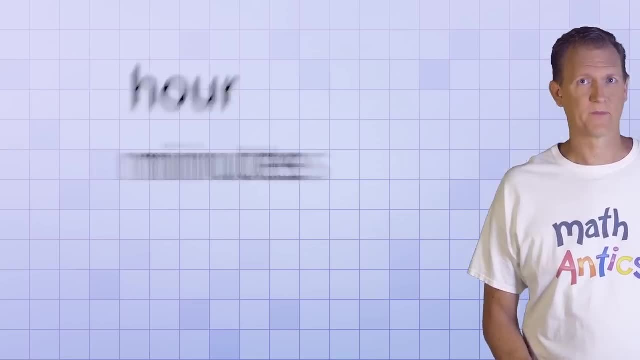 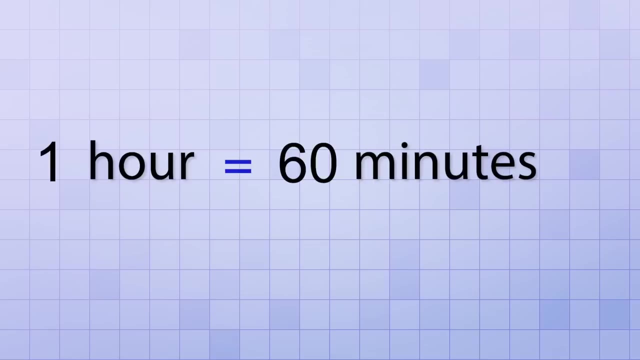 So we divide hours up into even smaller units, called minutes. Specifically, each hour is divided up into 60 minutes, So a minute is 1 60th of an hour. And to get even smaller units of time, we divide up each minute into 60 equal parts. 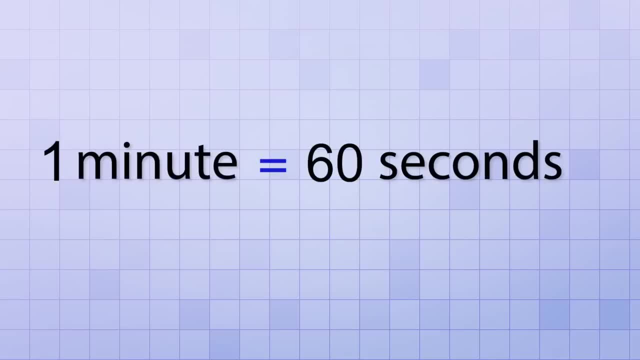 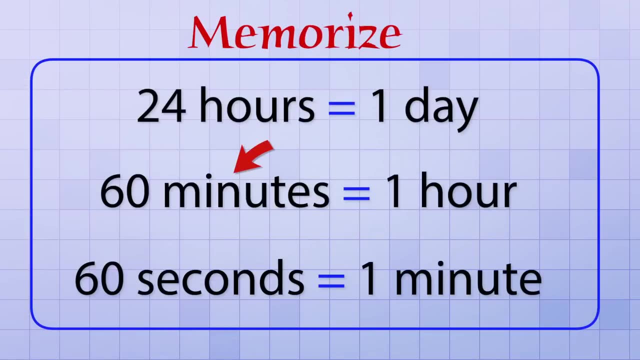 called seconds. So a second is 1 60th of a minute, Going from the smallest to the biggest. you should memorize that 60 seconds equals 1 minute, 60 minutes equals 1 hour and 24 hours equals 1 full day. 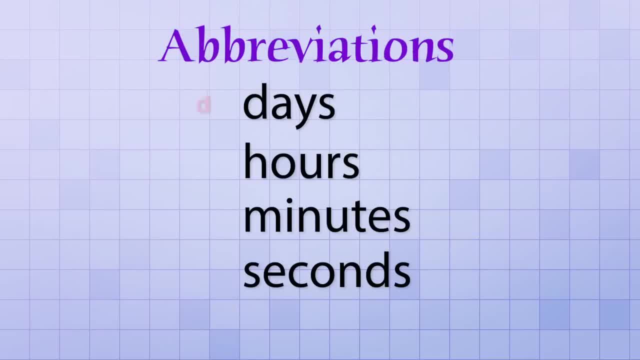 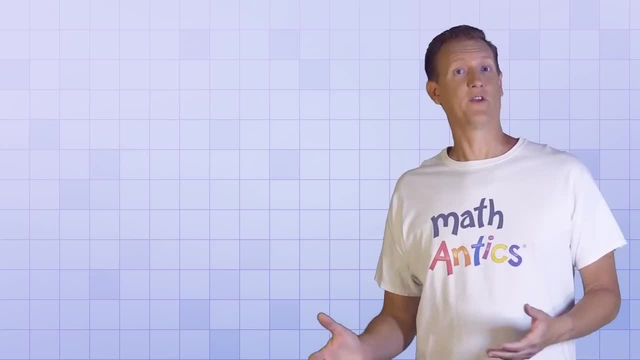 There are some common abbreviations for these units that you should know too: D for days, H for hours, min for minutes and s for seconds. One of the earliest devices for measuring time was called a sundial. It was basically a flat disk…. 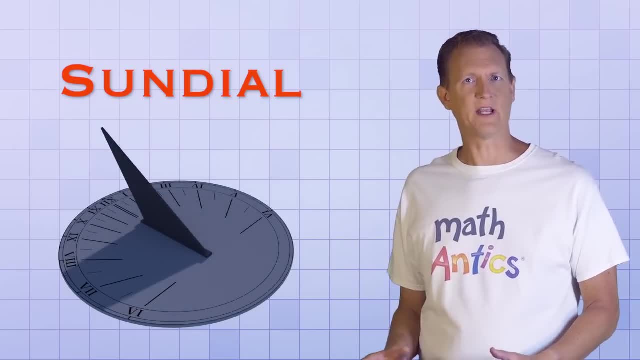 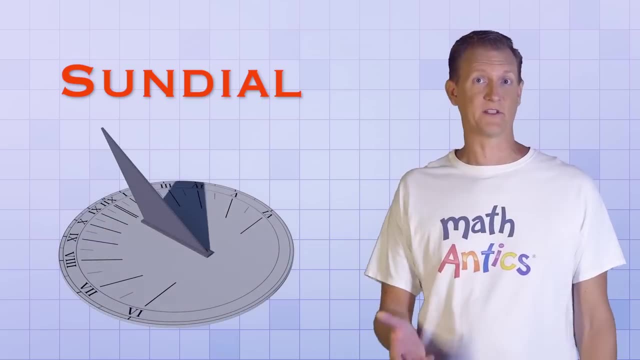 …with a triangular pointer in the middle. As the Earth rotated, the shadow of the pointer would slowly change position and point to different markings on the edge of the circle which represented different times of the day. Are you tired of the man telling you what time it is? 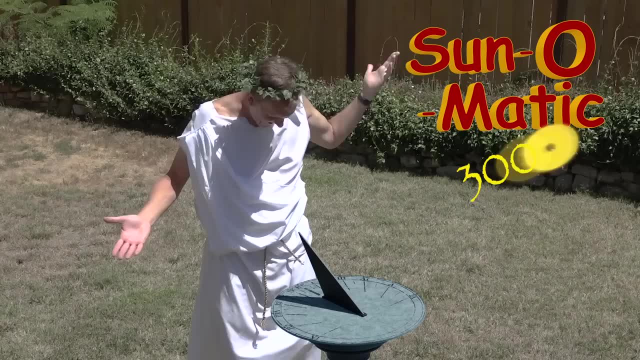 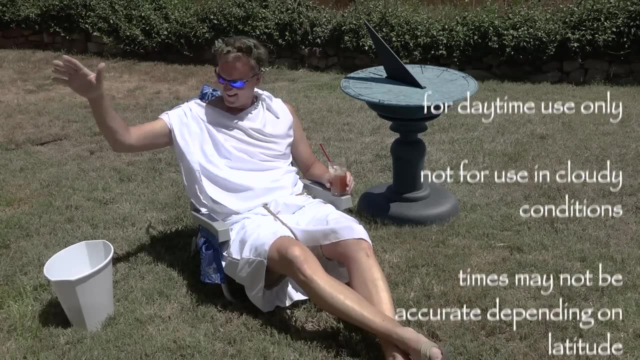 Now you can get the time directly from the source with the Sun-O-Matic 3000.. Just put it in your yard and let the sun do the rest. For daytime use only, not for use in cloudy conditions. Times may not be accurate depending on latitude. 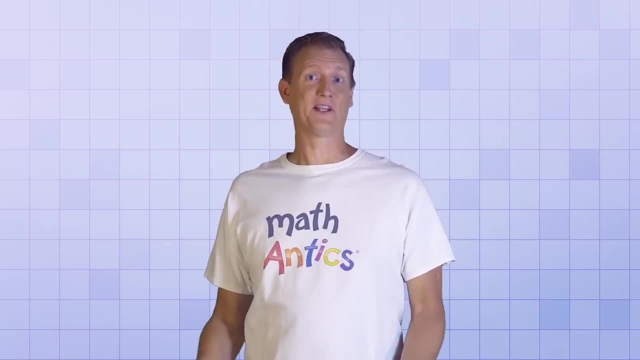 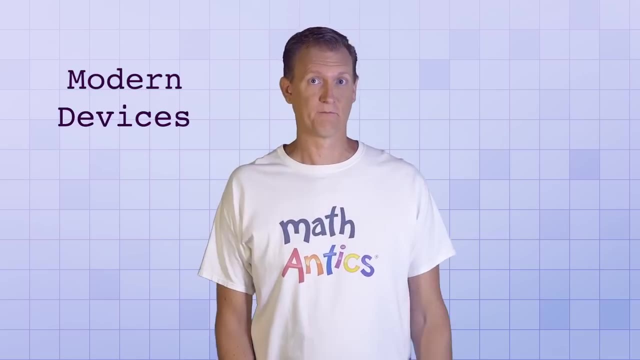 Some calibration required. The sundial was a really cool invention, but it had a lot of limitations. Fortunately, there are much better, modern devices for keeping track of time. In fact, you probably have one hanging on your wall at home or in your classroom that looks. 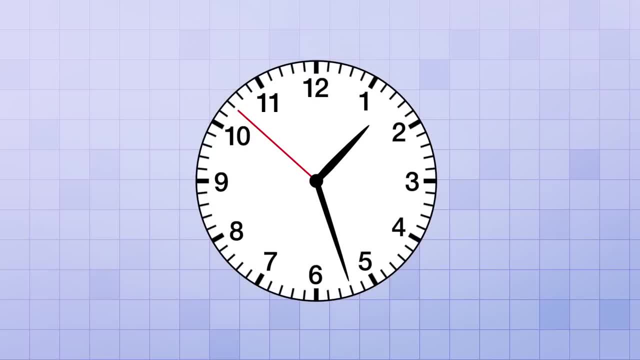 something like this. This traditional clock is designed to keep track of three different units of time: Seconds, minutes and hours. That's why it has three different pointers or hands. This thin red pointer is called the second hand because it helps us keep track of seconds. 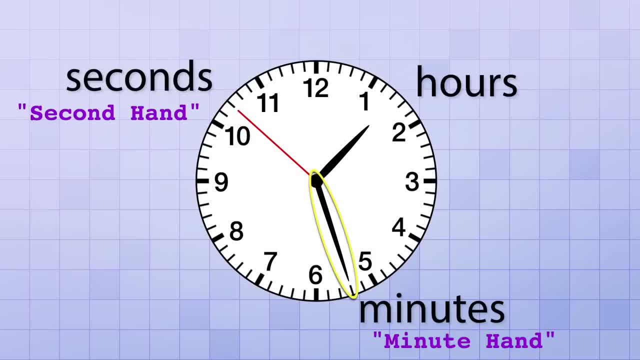 seconds. This thicker black pointer is called the minute hand because it helps us keep track of minutes, And this shorter black pointer is called the hour hand because it helps us keep track of hours. Oh, and the circle itself is often referred to as the clock face. 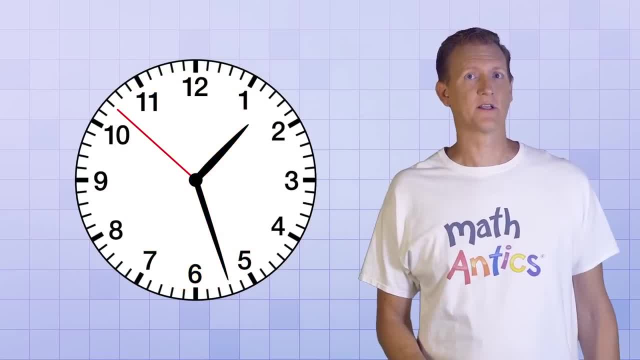 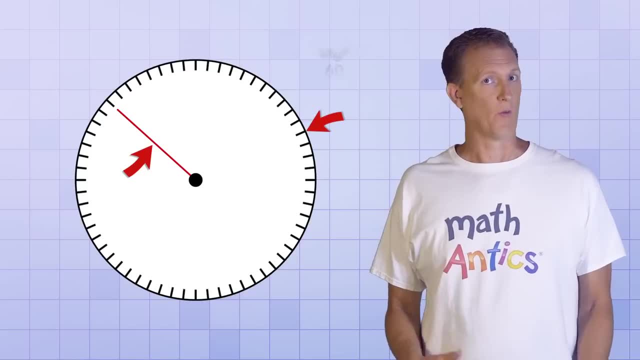 A clock is actually kinda complicated, So to see how it works, let's start with a version that has everything removed except for the second hand and the 60 marks around the edge of the clock face. Why are there 60 marks around the edge? 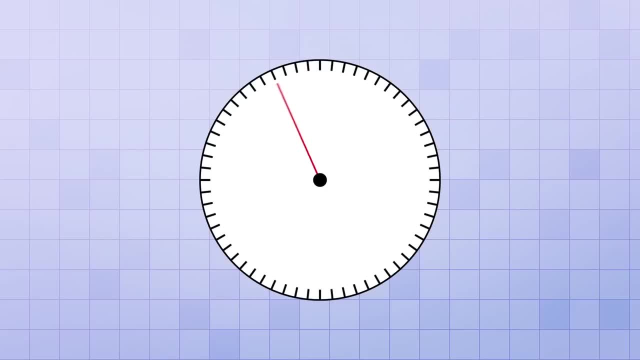 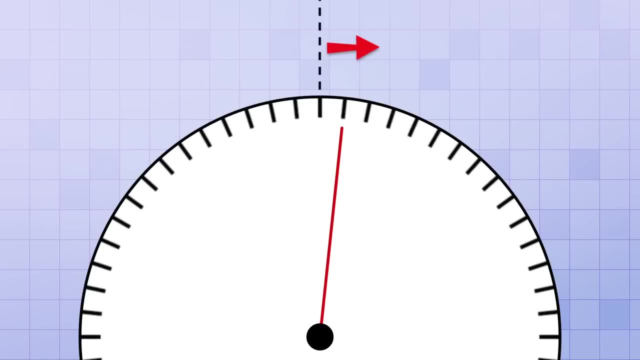 You'll see in just a minute, Starting with the second hand pointing straight up at the top of the clock face. if the hand rotates to the right so that it's pointing at the next mark, that means that 1 second of time has passed. so we'll label that mark 1.. 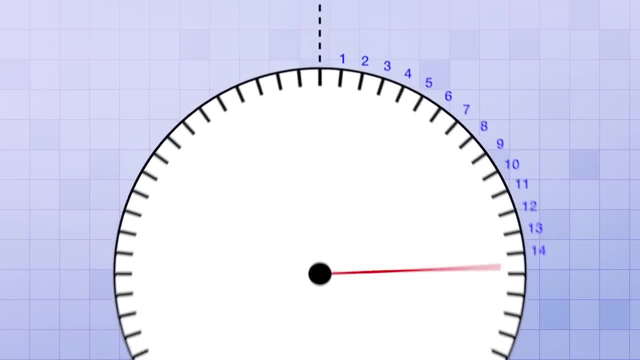 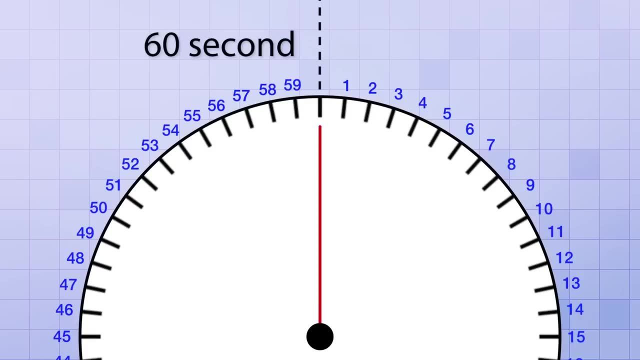 The next mark will be 2,, the next 3, and so on until we get all the way around and the hand is pointing straight up again. That means exactly 60 seconds have passed, so we'll label that mark with a 60.. 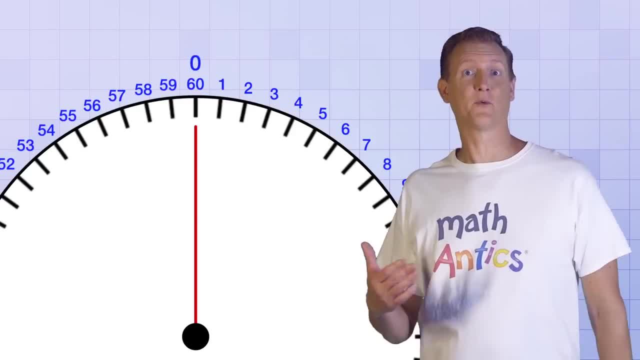 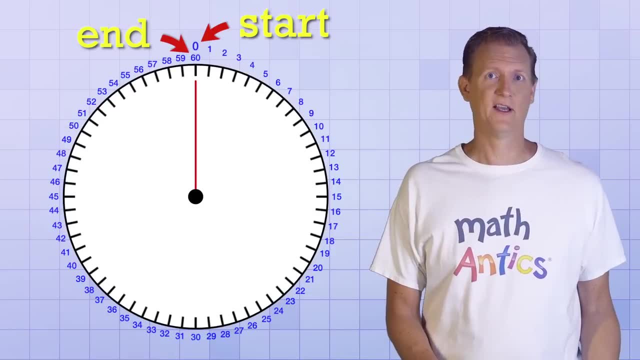 But we COULD have labeled that top mark as a 0. Since that's where the sequence of numbers starts. that's one of the cool things about a clock being a circle: The starting point is also the ending point, So as soon as you hit the end, you're also back at the beginning. 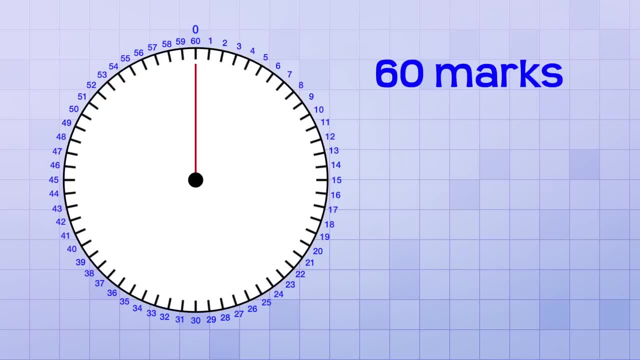 The reason that there's exactly 60 marks around the edge of a clock is that 60 seconds equals 1 minute. That means when the second hand makes one full rotation around the clock face, exactly 1 minute of time has passed, And if it makes 2 full rotations, 2 minutes have passed. 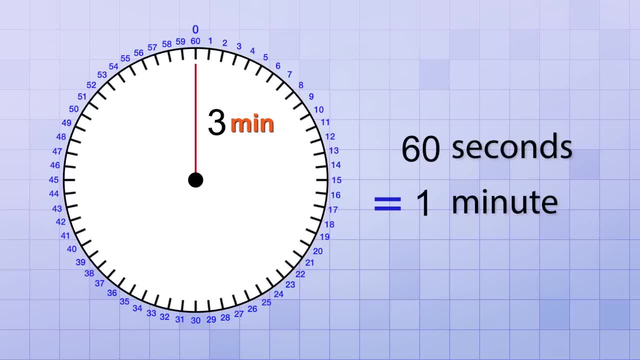 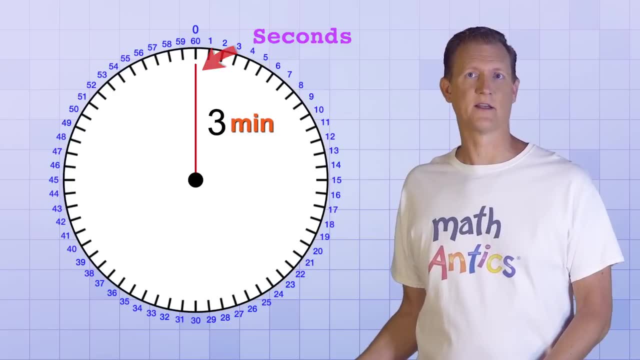 And if it makes 3 rotations, 3 minutes have passed, And so on. So, even though the second hand is counting seconds, it also helps us know how many minutes have passed. But how are we going to keep track of those minutes? 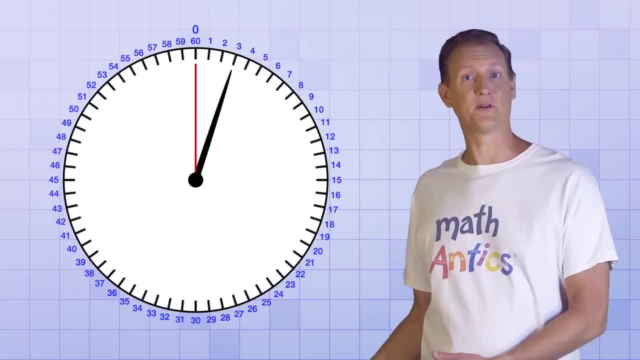 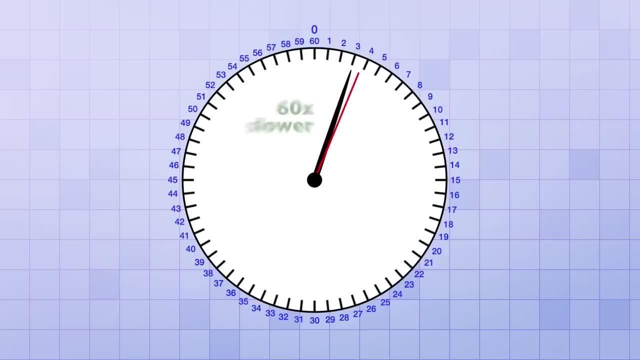 Well, that's where the minute hand comes in handy, So let's add it back to our simple clock. The minute hand works a lot like the second hand. The main difference is that it travels slower… 60 times slower, to be exact, Since a minute is 60 times longer than a second…. 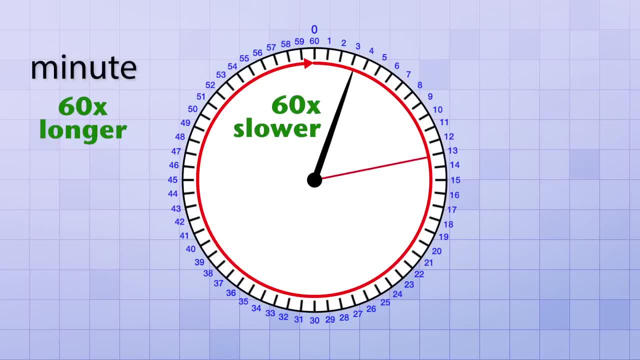 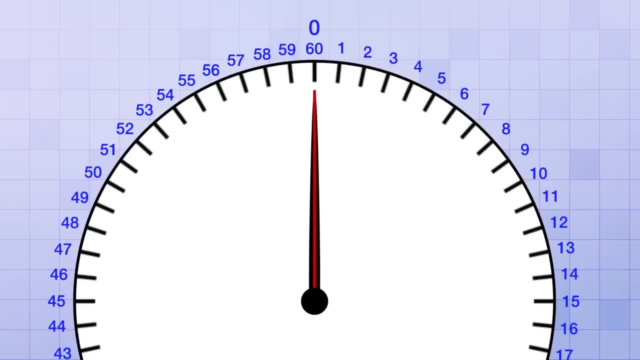 While the second hand travels all the way around the clock, the minute hand only moves from one mark to the next, For example, if both hands start straight up at the top of the clock, while the second hand travels all the way around the clock, counting out 60 seconds. as it goes the minute. 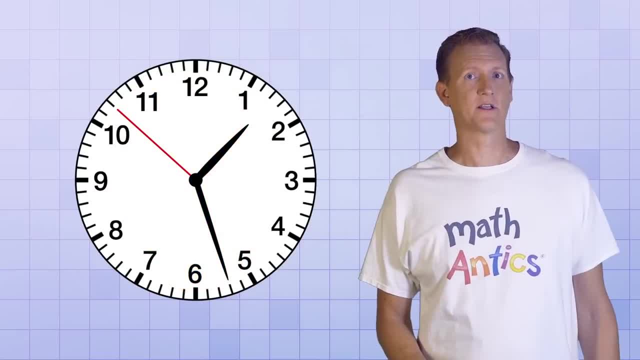 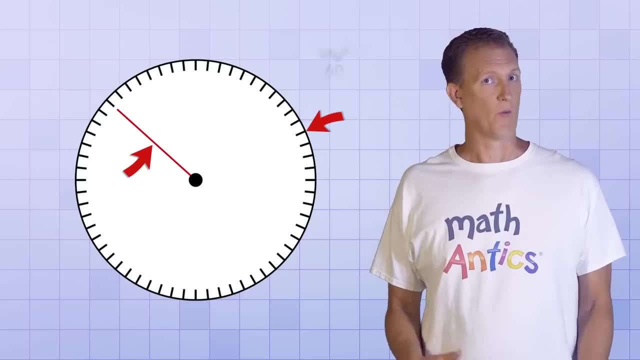 A clock is actually kind of complicated, So to see how it works, let's start with a version that has everything removed except for the second hand and the 60 marks around the edge of the clock face. Why are there 60 marks around the edge? 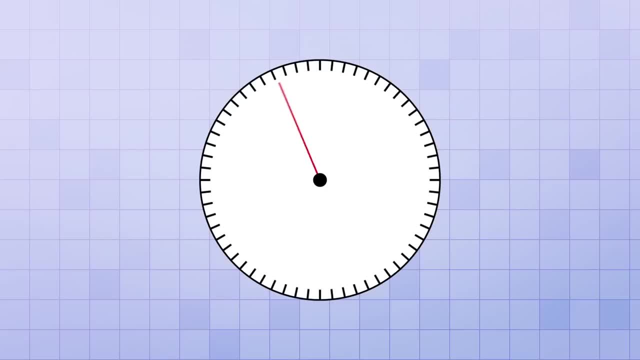 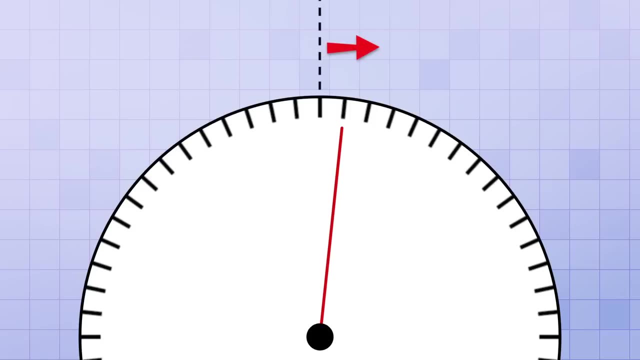 You'll see in just a minute, Starting with the second hand pointing straight up at the top of the clock face. if the hand rotates to the right so that it's pointing at the next mark, that means that 1 second of time has passed. so we'll label that mark 1.. 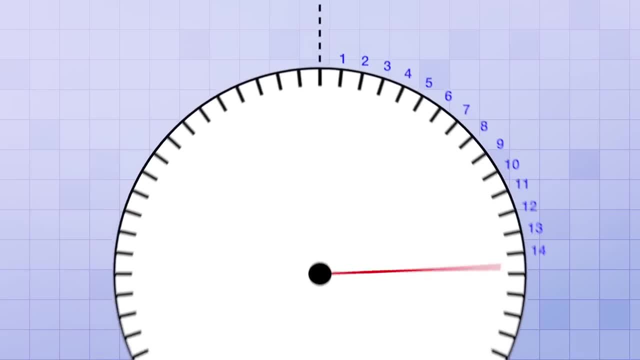 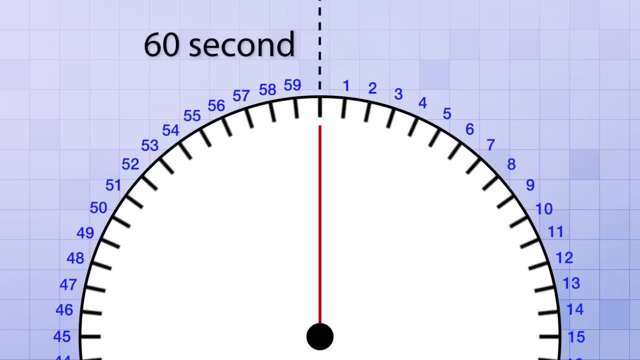 The next mark will be 2,, the next 3, and so on until we get all the way around and the hand is pointing straight up again. That means exactly 60 seconds have passed, so we'll label that mark with a 60.. 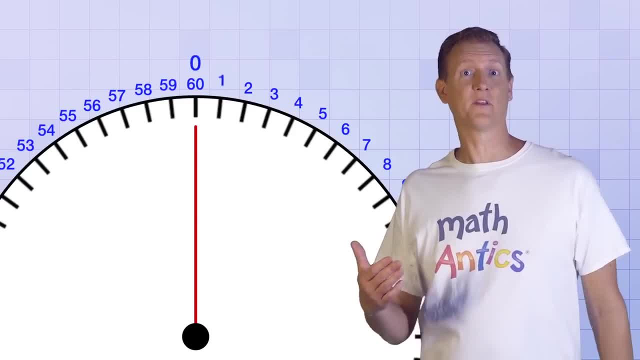 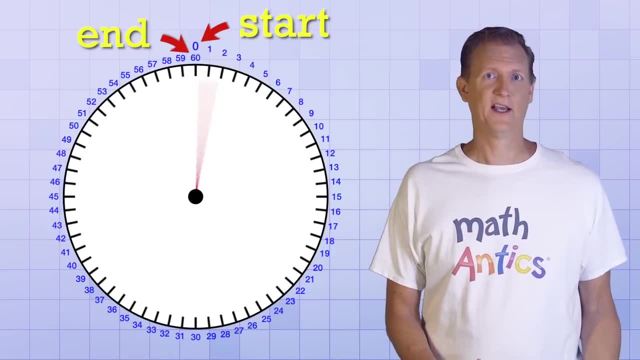 But we could have labeled that top mark as a 0. Since that's where the sequence of numbers starts. that's one of the cool things about a clock being a circle: The starting point is also the ending point, So as soon as you hit the end, you're also back at the beginning. 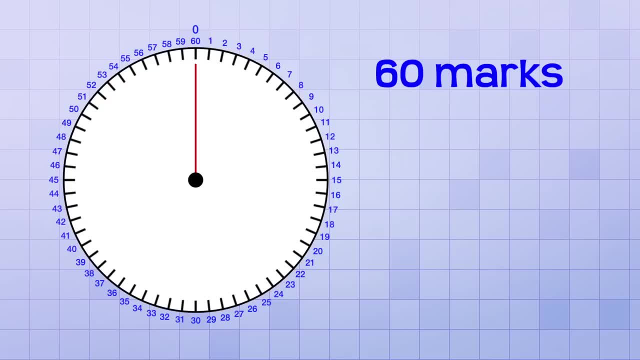 The reason that there's exactly 60 marks around the edge of a clock is that 60 seconds equals 1 minute. That means when the second hand makes one full rotation around the clock face, exactly 1 minute of time has passed, And if it makes 2 full rotations, 2 minutes have passed. 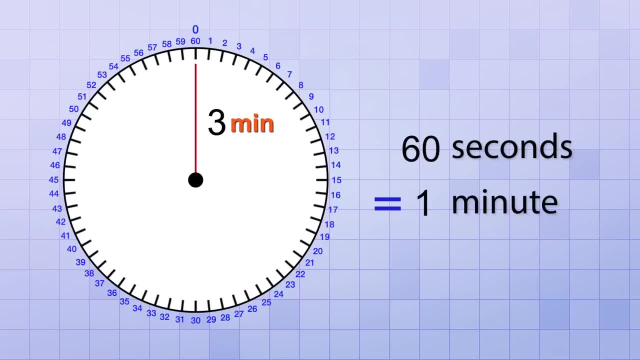 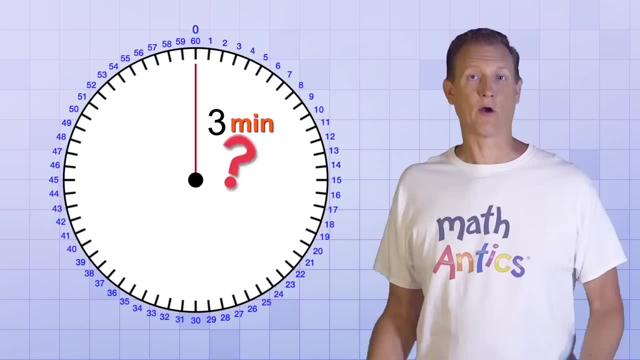 And if it makes 3 rotations, 3 minutes have passed, And so on. So, even though the second hand is counting seconds, it also helps us know how many minutes have passed. But how are we going to keep track of those minutes? 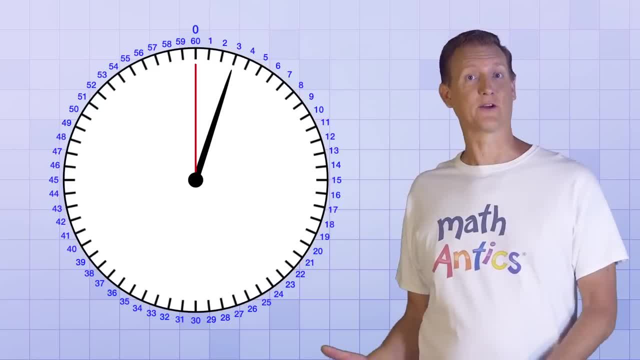 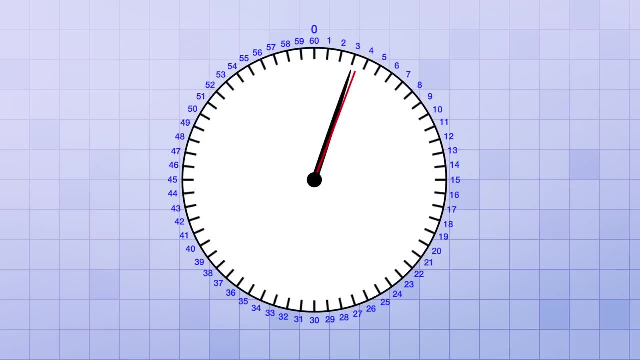 Well, that's where the minute hand comes in handy, So let's add it back to our simple clock. The minute hand works a lot like the second hand. The main difference is that it travels slower… 60 times slower, to be exact, Since a minute is 60 times longer than a second. 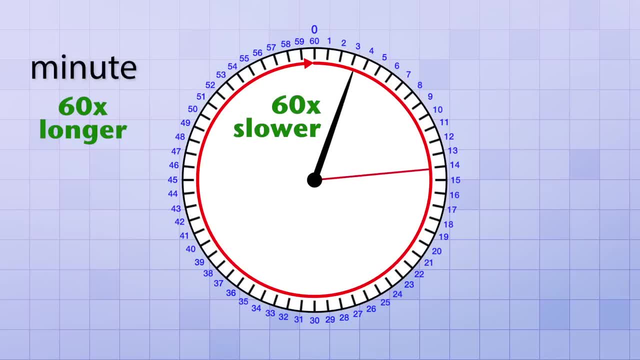 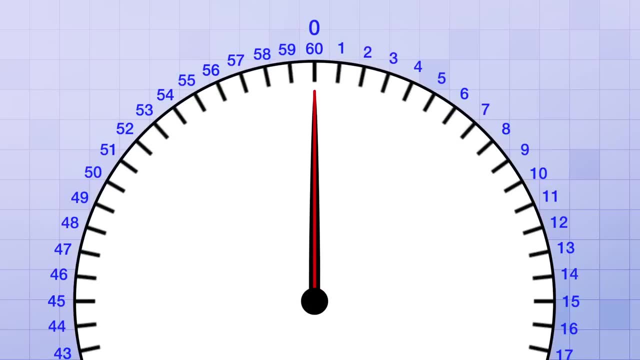 the minute hand only moves from one mark to the next. For example, if both hands start straight up at the top of the clock, while the second hand travels all the way around the clock, counting out 60 seconds as it goes the minute. 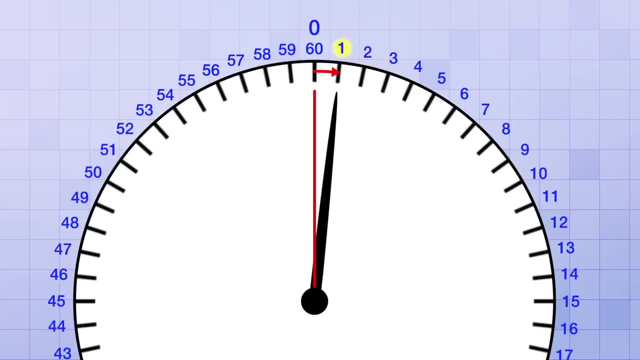 hand will only travel from 0 to 1, because only 1 minute has passed. Then, while the second hand travels around the clock a second time, the minute hand will travel from 1 to 2, because 2 minutes have passed. 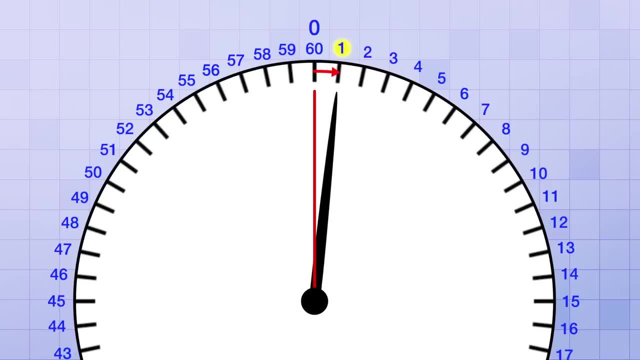 hand will only travel from 0 to 1. Because only 1 minute has passed. Then, while the second hand travels around the clock a second time, the minute hand will travel from 1 to 2. Since 2 minutes have passed. 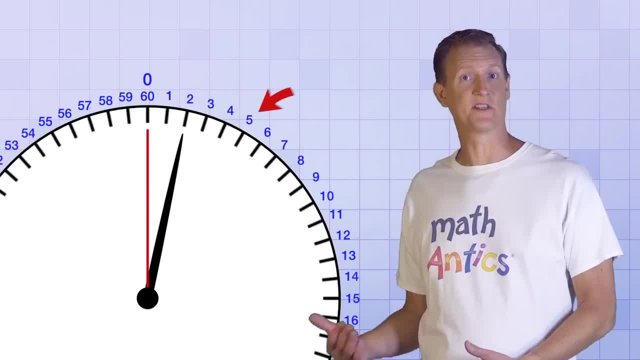 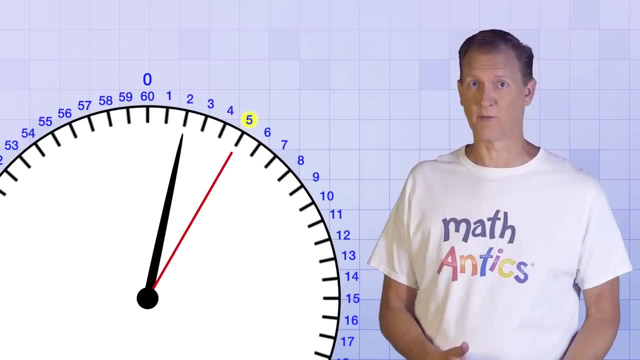 Notice that we use the exact same set of 60 marks to measure both seconds and minutes, But the different hands tell you how to interpret those marks. If the second hand is pointing at the 5th mark, it means 5 seconds, But if the minute hand is pointing at the 5th mark, it means 5 minutes. 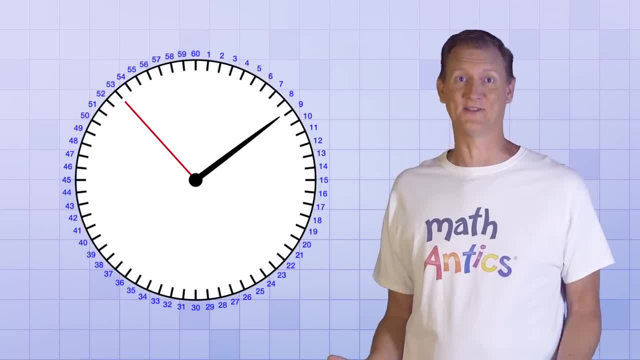 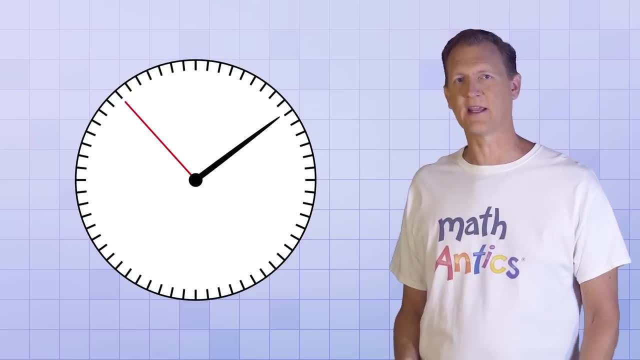 Of course, being able to quickly tell which mark a hand is pointing at is tricky, since clocks don't usually number every mark. So to make it easier, the inventors of the clock decided to make every 5th mark bigger or bolder, so you could skip count by 5s, which helps you quickly. 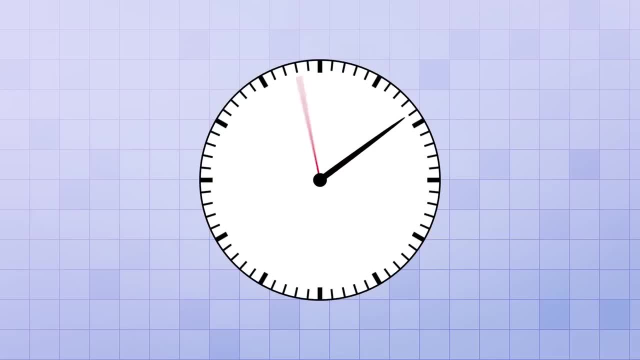 tell where the hands are pointing. For example, if the second hand is pointing right here, you can tell right away that it's just 2 marks past the 15th mark. so it's pointing at 17 seconds, since 15 plus 2 equals 17.. 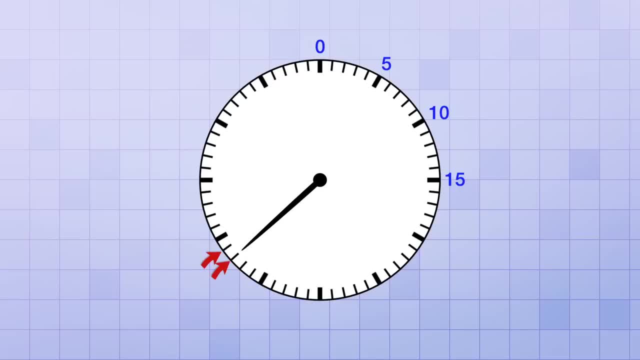 And if the minute hand is pointing here, you'll quickly see that it's just 2 marks before the 40th mark, so it's pointing to 38 minutes, since 40 minus 2 equals 38.. These bigger marks are so helpful for reading a clock that you should memorize the values. 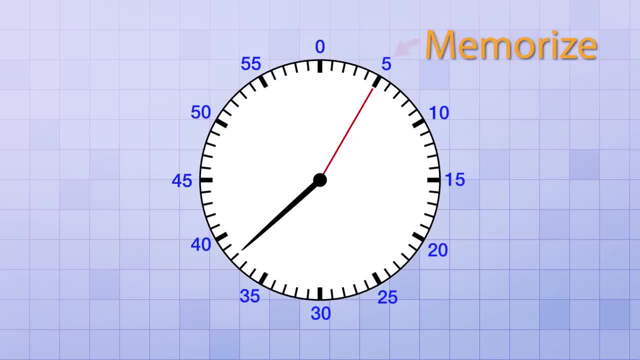 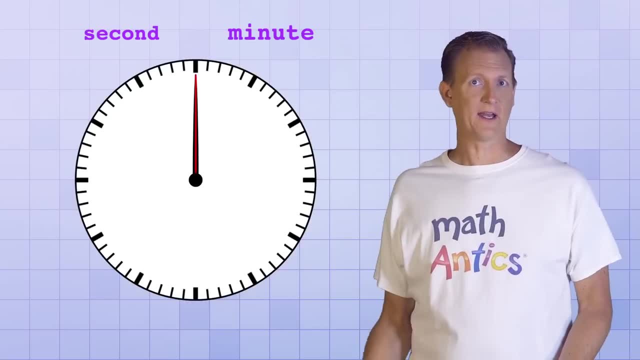 they represent when the minute or second hands are pointing at them, especially the ones that break the clock face up into quarters. OK, so now you know how the second and minute hands work. When the second hand goes all the way around, the minute hand increases by 1.. 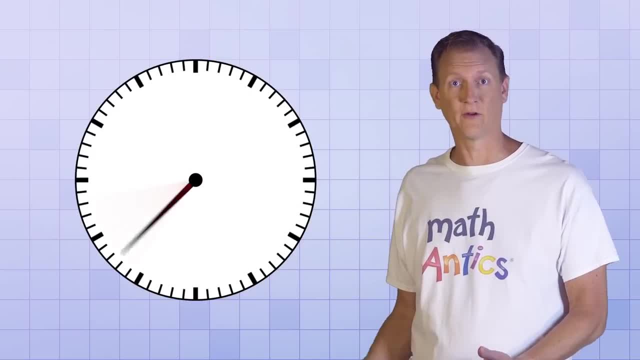 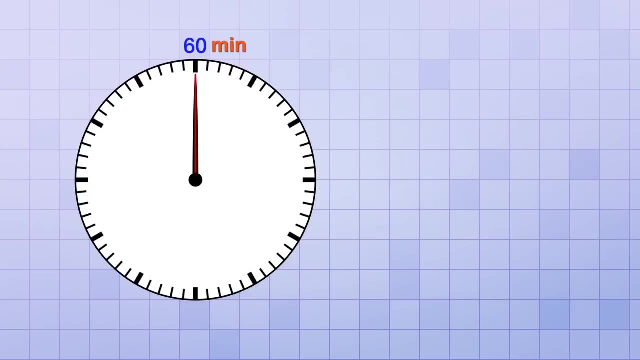 But what happens when the minute hand eventually goes all the way around and is counted out 60 minutes? If you paid close attention at the beginning of the video, you probably know what that means. 60 minutes equals 1 hour, So when the minute hand goes all the way around, it means 1 hour of time has passed. 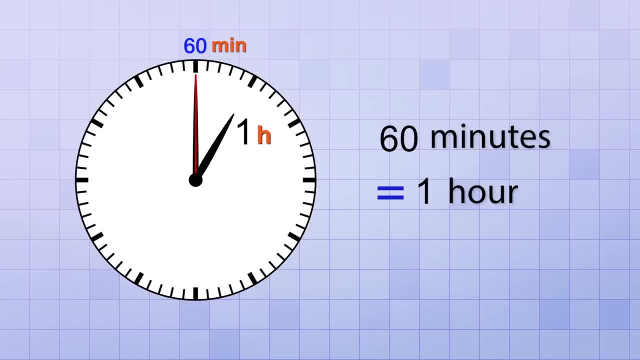 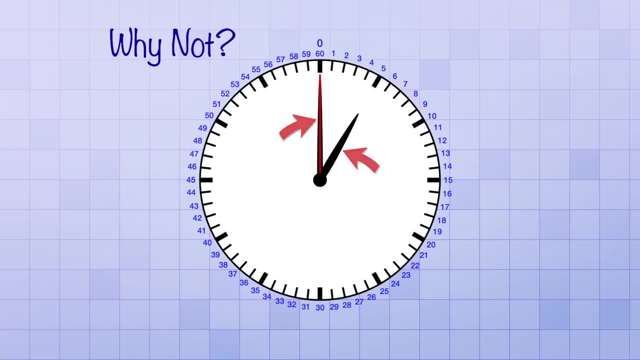 That means we're going to need to add the hour hand back to our clock to keep track of hours. But the hour hand doesn't use the 60 marks on the edge of the clock in the same way that the other hands do. Why not? 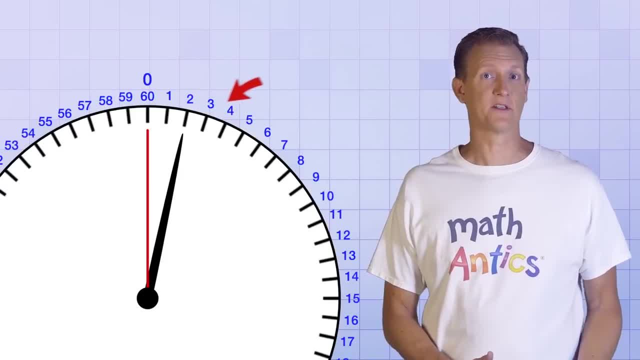 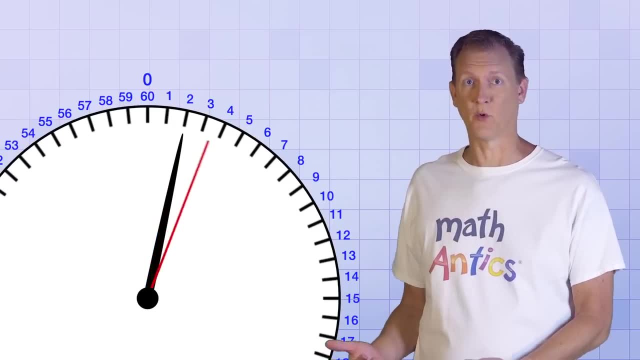 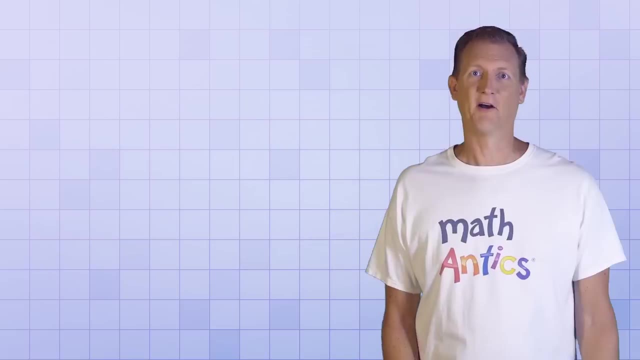 Notice that we use the exact same set of 60 marks to measure both seconds and minutes, But the different hands tell you how to interpret those marks. If the second hand is pointing at the fifth mark, it means 5 seconds, But if the minute hand is pointing at the fifth mark, it means 5 minutes. 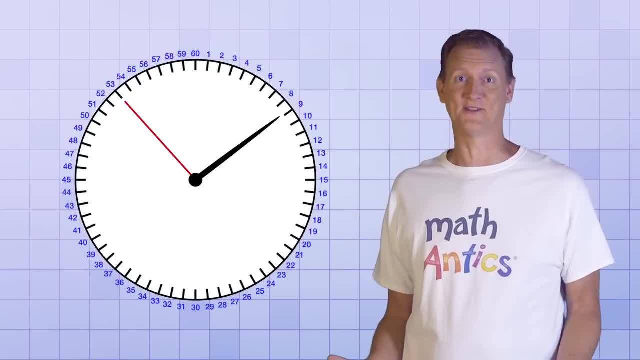 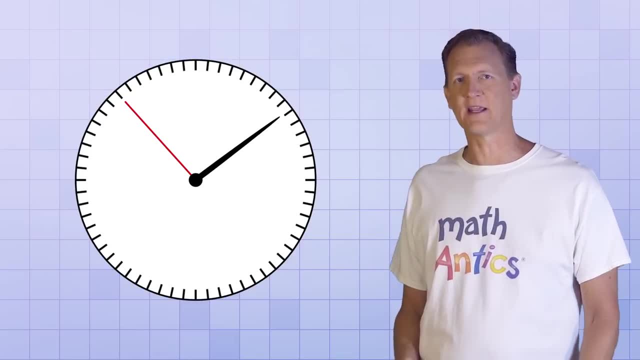 Of course, being able to quickly tell which mark a hand is pointing at is tricky, since clocks don't usually number every mark. So to make it easier, the inventors of the clock decided to make every fifth mark bigger or bolder, so you could skip count by fives, which helps you quickly tell where the hands. 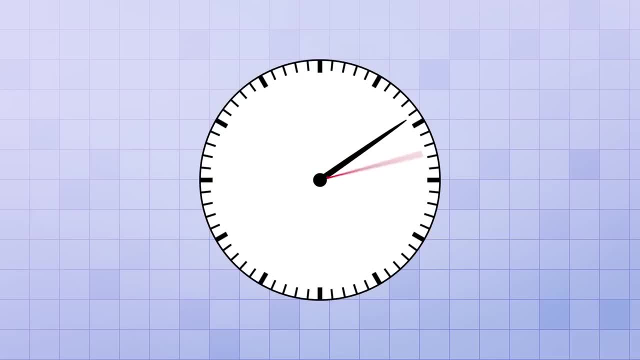 are pointing. For example, if the second hand is pointing right here, you can tell right away that it's just 2 marks past the 15th mark. so it's pointing at 17 seconds, since 15 plus 2 equals 17.. 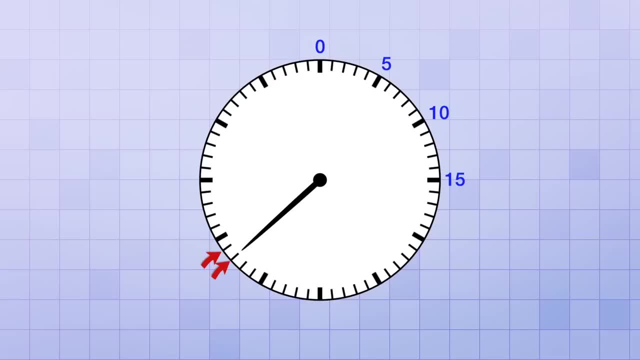 And if the minute hand is pointing here, you'll quickly see that it's just 2 marks before the 40th mark. so it's pointing to 38 minutes, since 40 minus 2 equals 38.. These bigger marks are smaller. 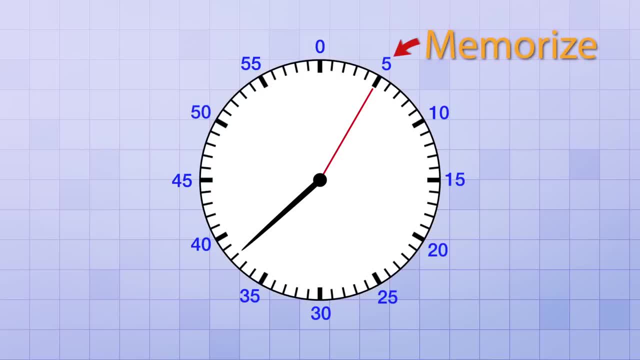 They're so helpful for reading a clock that you should memorize the values they represent when the minute or second hands are pointing at them, especially the ones that break the clock face up into quarters. OK, so now you know how the second and minute hands work. 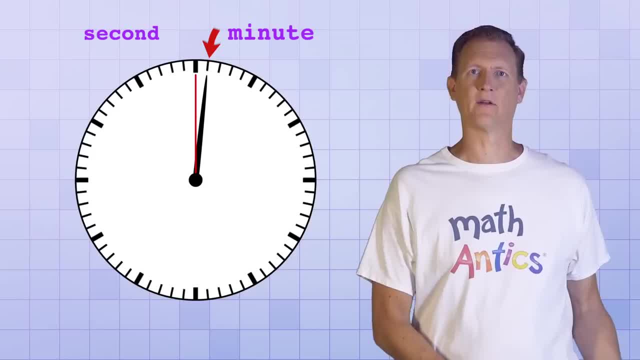 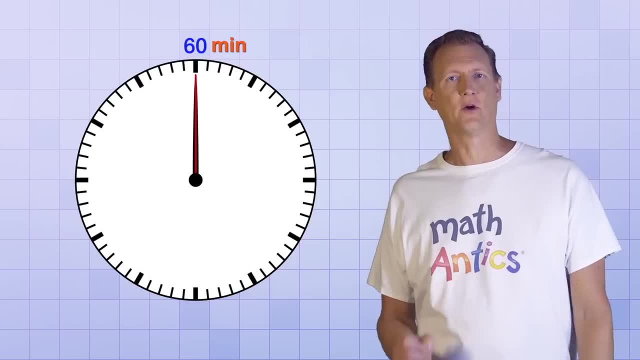 When the second hand goes all the way around, the minute hand increases by 1.. But what happens when the minute hand eventually goes all the way around and has counted out 60 minutes? If you paid close attention at the beginning of the video, you probably know the answer. 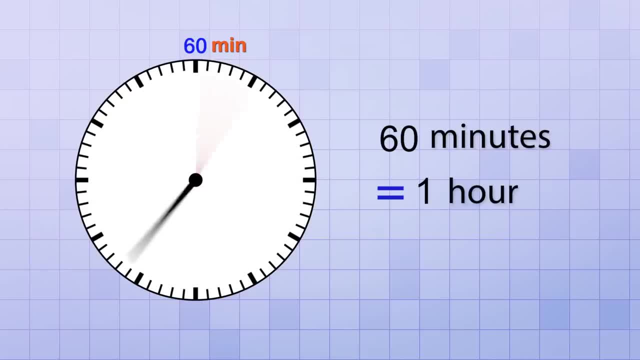 60 minutes equals 1 hour, So when the minute hand goes all the way around, it means 1 hour of time has passed. That means we're going to need to add the hour hand back to our clock to keep track of hours. 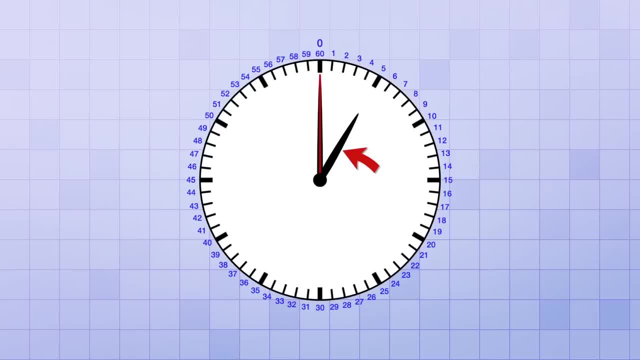 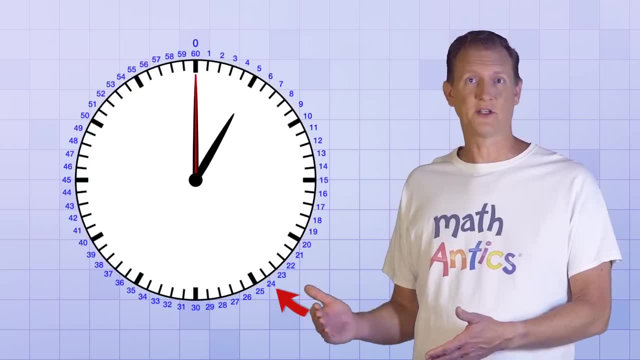 But the hour hand doesn't use the 60 marks on the edge of the clock in the same way that the other hands do. Why not? Because there aren't 60 hours in a day, There's only 24.. If the hour hand just moved 1 mark for each hour, it wouldn't make it all the way around. 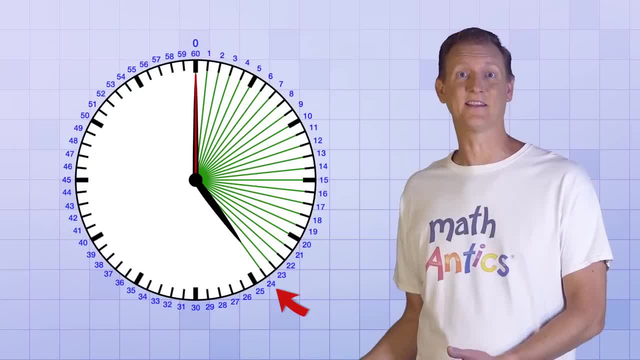 the clock face in a single day. Ideally, it would be nice if we could have a clock face on the edge of the clock face. It would be nice if we could have a clock face on the edge of the clock face in a single day. 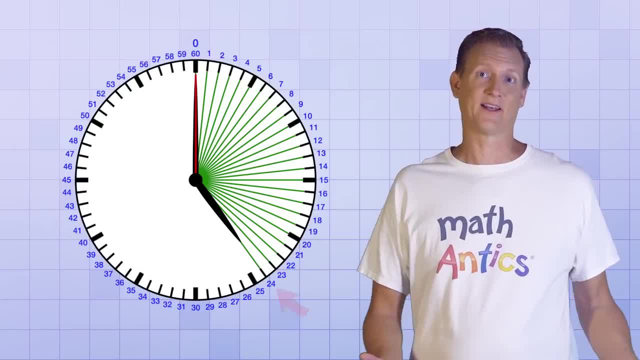 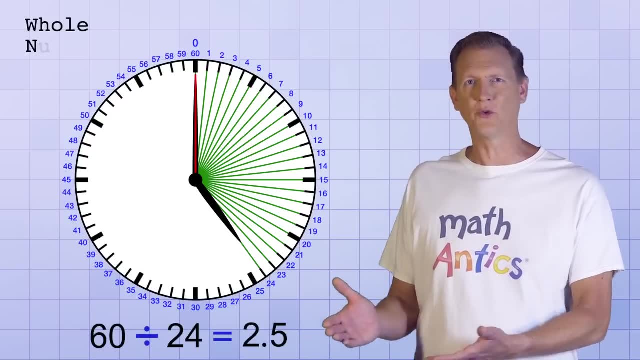 Unfortunately we could have the hour hand go around the clock once per day. But unfortunately the 60 marks on the clock don't divide evenly by 24.. That means you can't find a nice whole number to skip. count to 24 by. 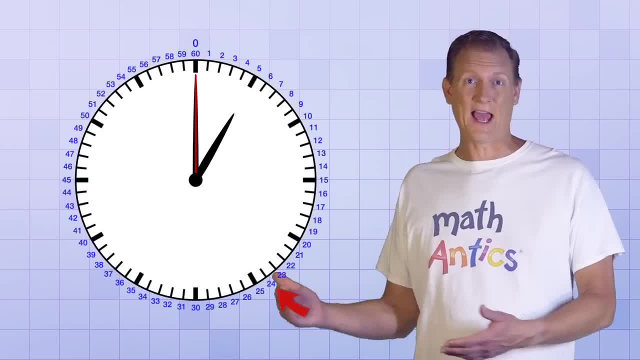 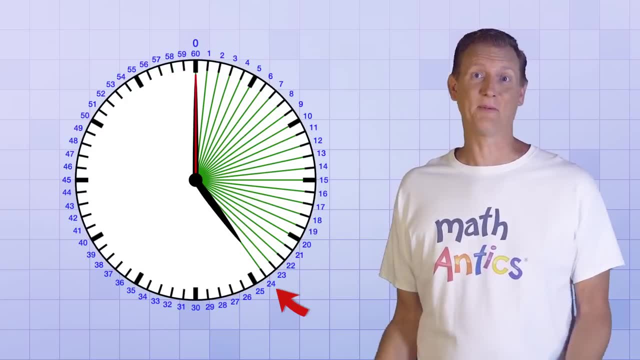 Because there aren't 60 hours in a day, there's only 24.. If the hour hand just moved 1 mark for each hour, it wouldn't make it all the way around the clock face in a single day. It would be nice if we could have the hour hand go around the clock once per day. 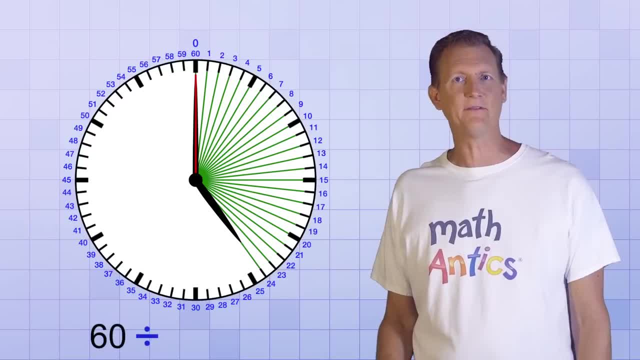 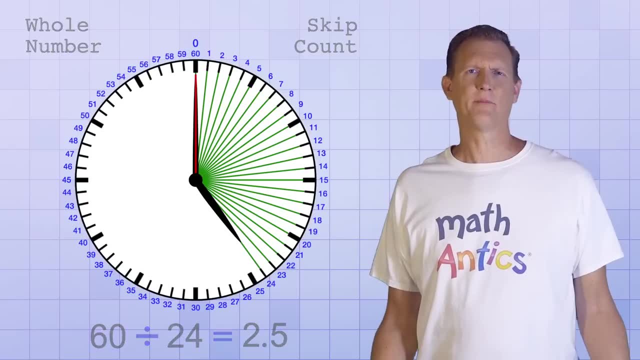 But unfortunately the 60 marks on the clock don't divide evenly by 24.. That means you can't find a nice whole number to skip count to 24 by. For example, if you had the hour hand move 2 marks for each hour, it still wouldn't. 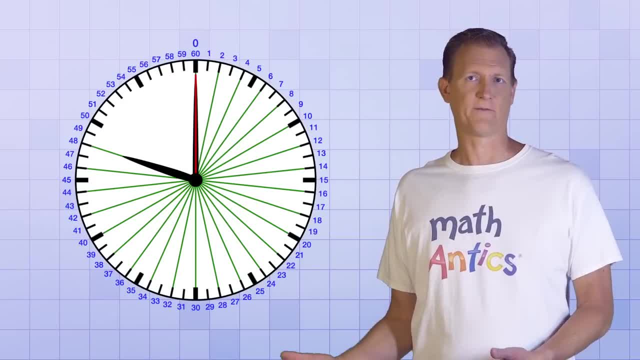 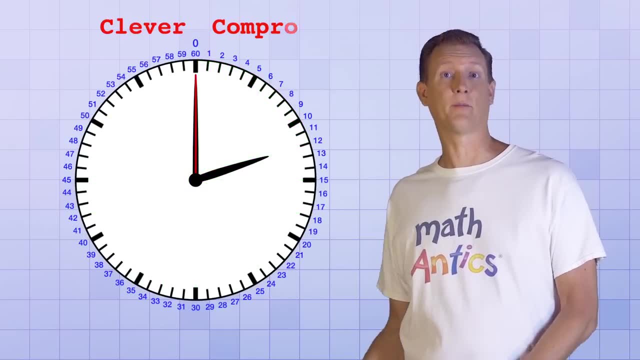 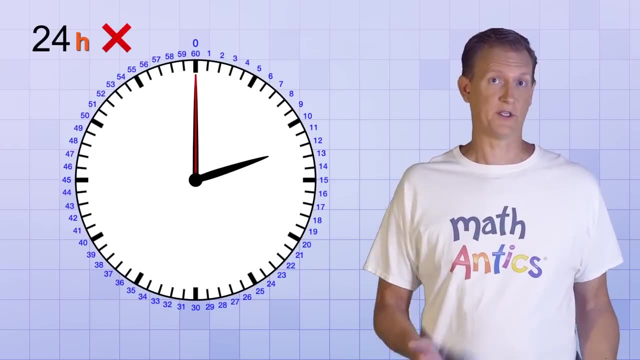 go far enough to make it all the way around the clock in a day, And if you had it move 3 marks for each hour, it would go too far. Fortunately, the inventors of the clock came up with a clever compromise. They realized that even though 24 hours doesn't divide evenly into 60, half of a day, which 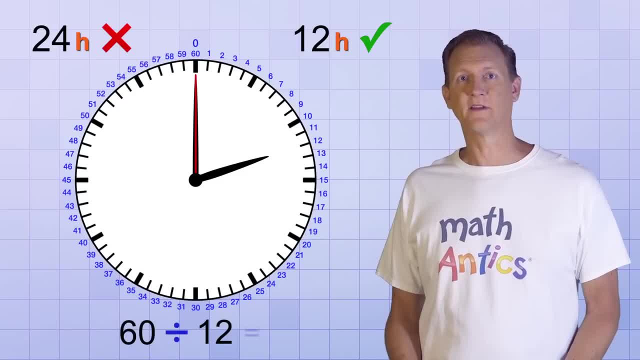 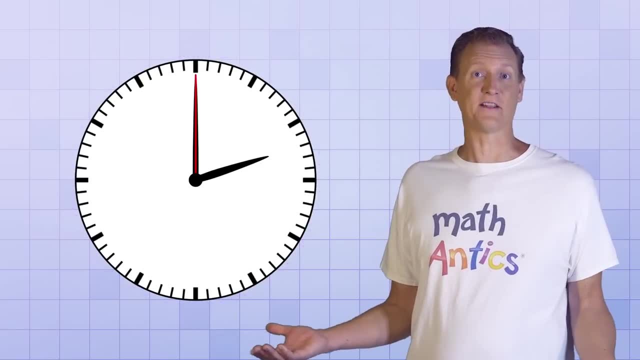 is 12 hours does. 60? divided by 12 equals 5. And 5 is a nice whole number to skip count by. In fact, we already have bigger marks on our clock face, every 5 marks, which makes this idea really convenient. 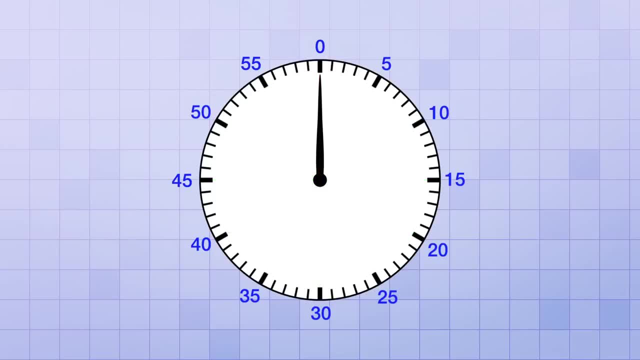 If the hour and minute hands start pointing straight up- as the minute hand goes all the way around, the clock- counting out 60 minutes… will slowly move past the first 5 marks, which means 1 hour has passed. Then, as the minute hand goes all the way around again, the hour hand will move past the next 5 marks. 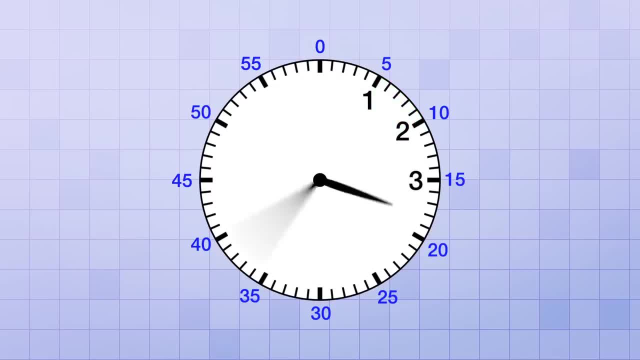 which means that 2 hours will have passed. This continues on until the hour hand makes it all the way around the clock and gets to the 12 hour mark back at the top. Just like with minutes and seconds, the top position on the clock represents both the beginning and the end of the counting sequence. 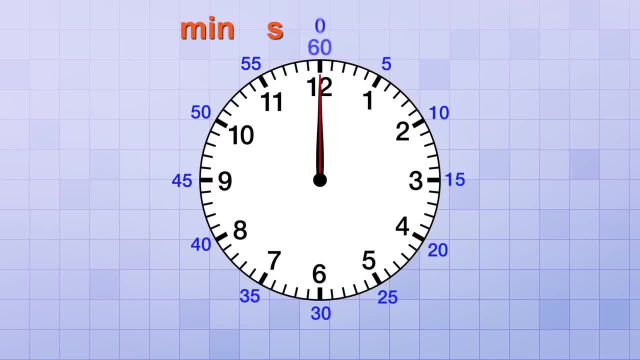 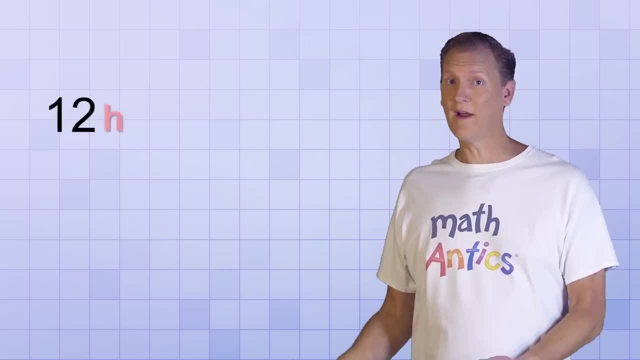 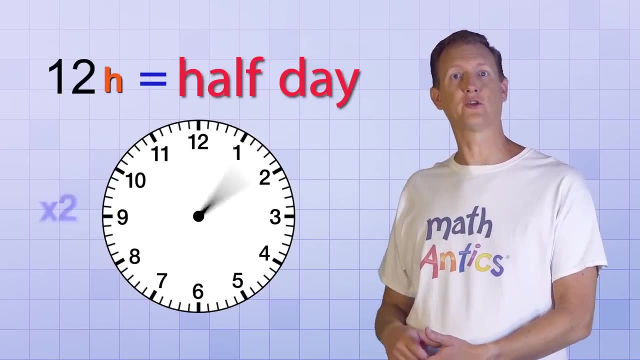 For minutes and seconds that means the top position represents both 60 and 0. But for the hour hand that top spot represents both 12 and 0.. Of course, 12 hours is only half the day. That means in order for this clock to keep track of one whole day, the hour hand needs to make 2 full trips around the clock face. 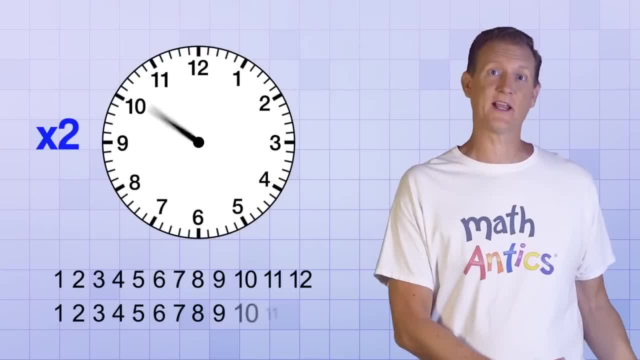 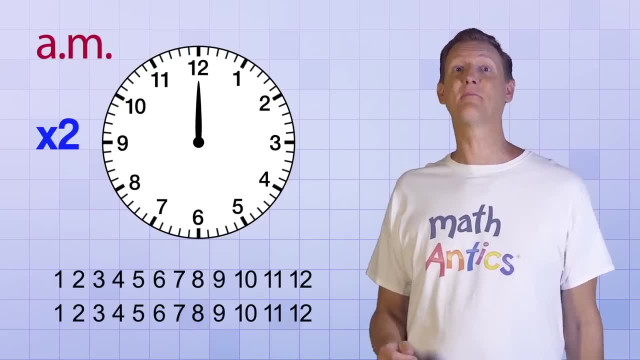 It counts out 12 hours- the first half, and then 12 more for the second half. That means that each hour mark is passed twice during the day, so we need a way to distinguish them, And that's where… AM and PM can help us out. 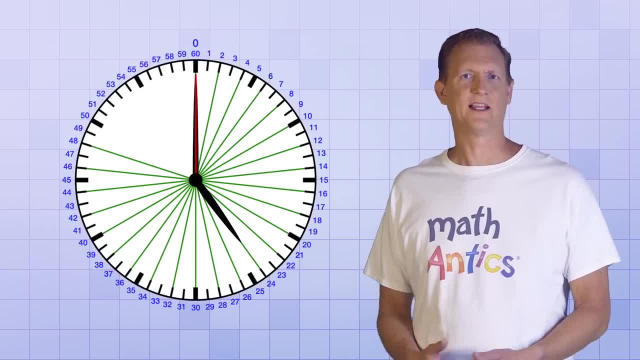 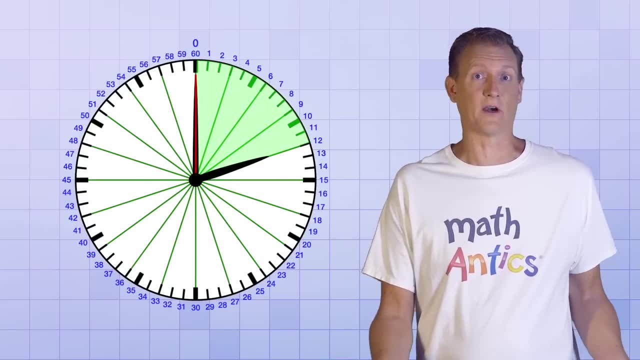 For example, if you had the hour hand move 2 marks for each hour, it still wouldn't go far enough to make it all the way around the clock in a day. And if you had it move 3 marks for each hour, it would go too far. 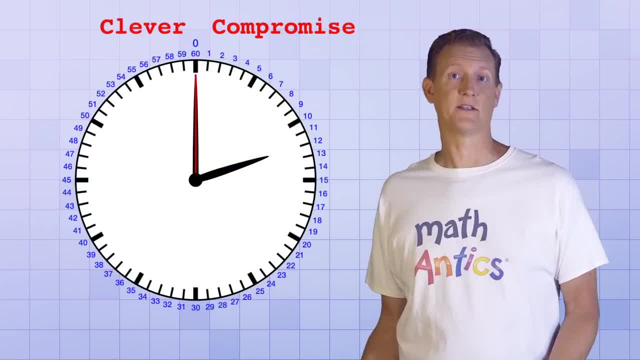 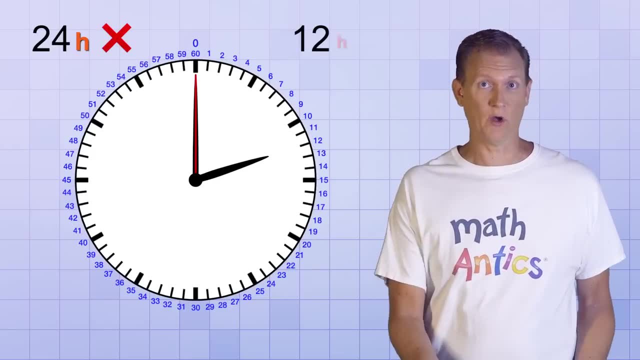 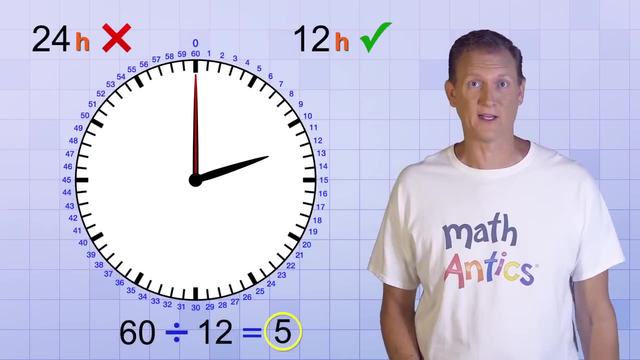 Fortunately, the inventors of the clock came up with a clever compromise. they realized that, even though 24 hours doesn't divide evenly into 60, half of a day does. 60 divided by 12 equals 5, and 5 is a nice whole number to skip count by. 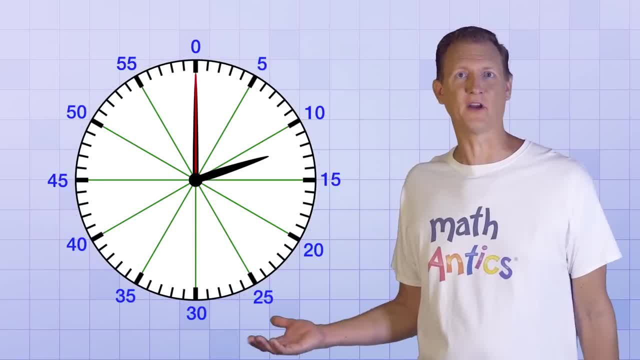 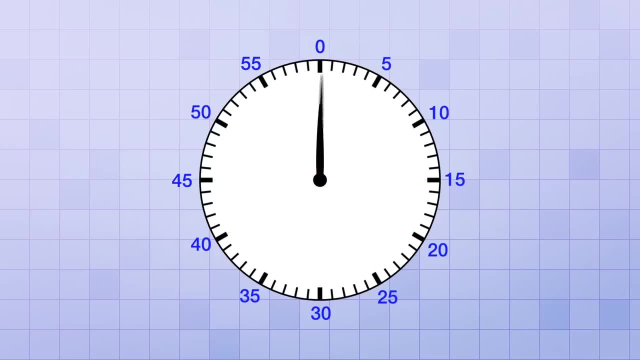 In fact, we already have bigger marks on our clock face- every 5 marks, which makes this idea really convenient If the hour and minute hands start pointing straight up as the minute hand goes all the way around the clock counting out 60 minutes. 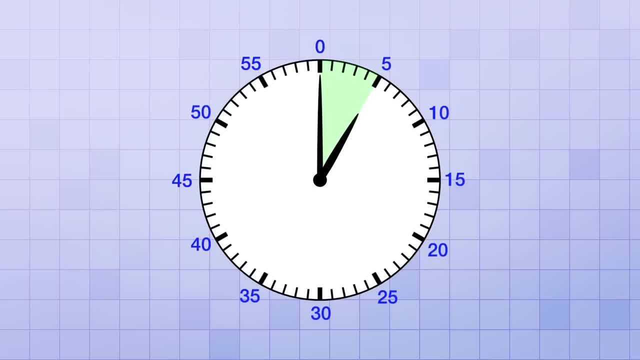 the hour hand will slowly move past the first 5 marks, which means 1 hour has passed. Then, as the minute hand goes all the way around again, the hour hand will move past the next 5 marks, which means that 2 hours will have passed. 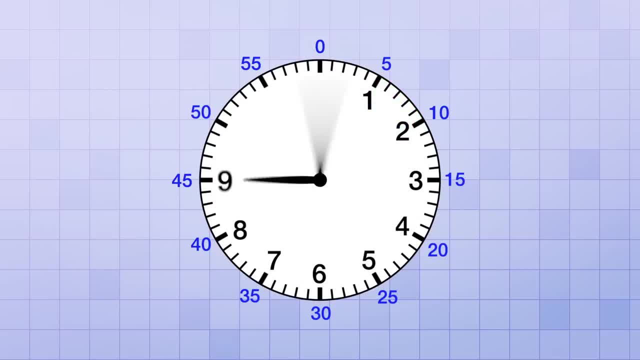 This continues on until the hour hand, makes it all the way around the clock and gets to the 12 hour mark back at the top. Just like with minutes and seconds, the top position on the clock represents both the beginning and the end of the counting sequence. 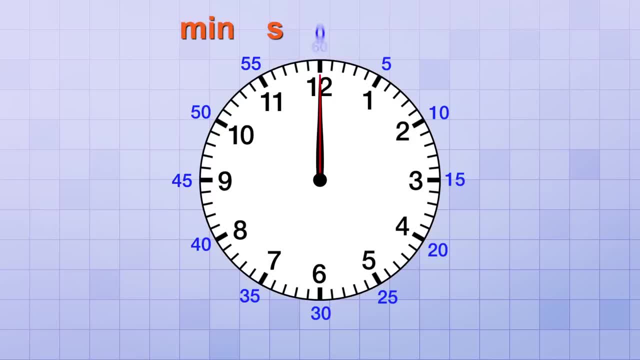 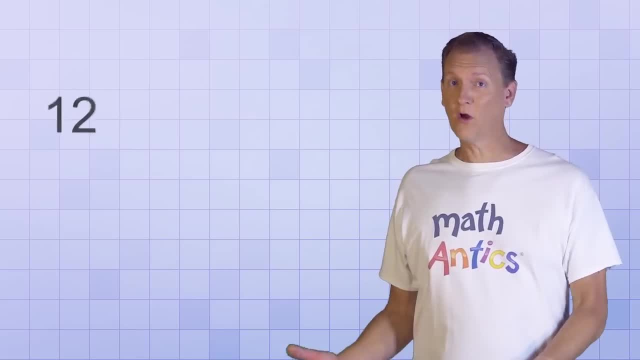 For minutes and seconds, that means the top position represents both 60 and 0. But for the hour hand, that top spot represents both 12 and 0.. Of course, 12 hours is only half a day. That means, in order for this clock to keep track of one whole day. 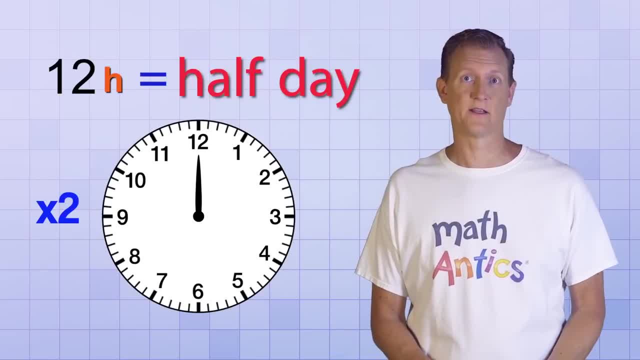 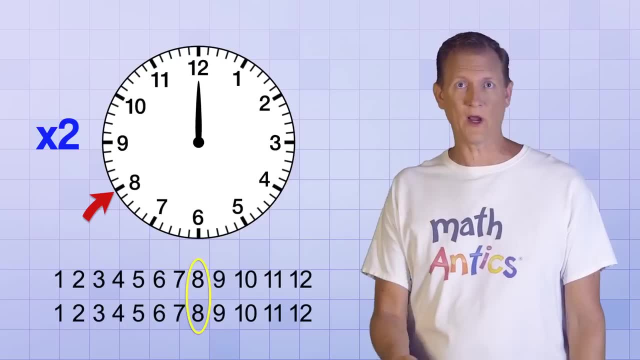 the hour hand needs to make two full trips around the clock face. It counts out 12 hours- the first half- and then 12 more for the second half. That means that each hour mark is passed twice during the day, so we need a way to distinguish them. 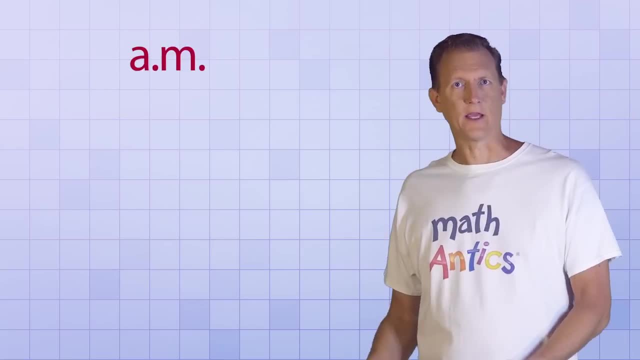 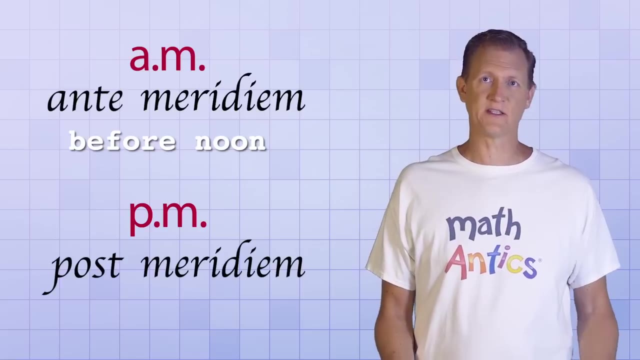 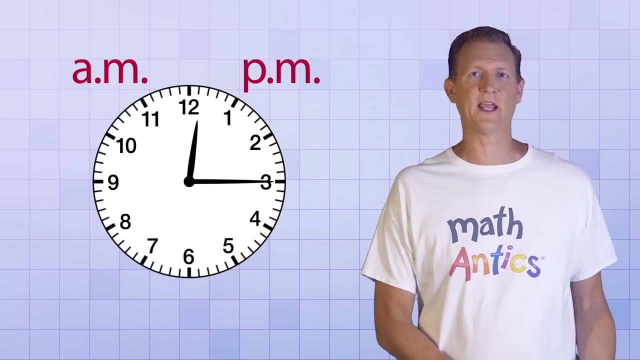 And that's where AM and PM can help us out. AM stands for Anti-Meridian, which just means Before Noon, And PM stands for Post-Meridian, which just means After Noon. To see how the AM and PM labels work with the 12 hours on our clock face to keep track of a full day. 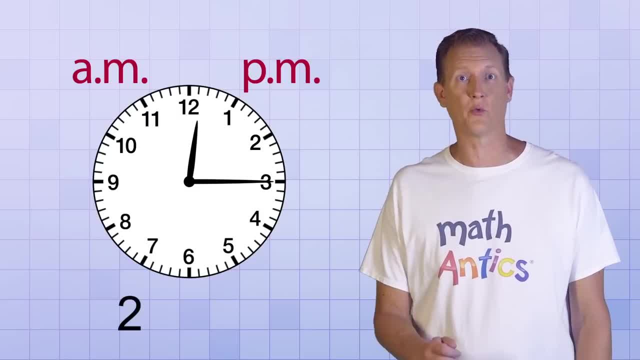 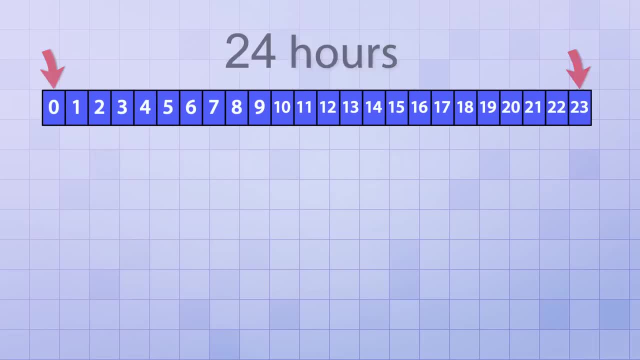 let's compare them to a simpler modern timekeeping system called the 24 hour clock. In that system, the 24 hours of the day are just labeled 0 through 23.. In other words, at the beginning of the day, which happens to be midnight. 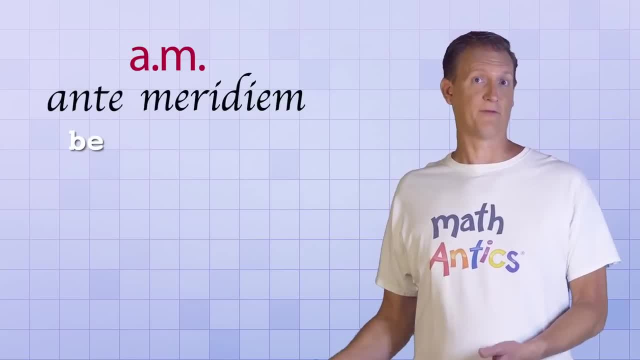 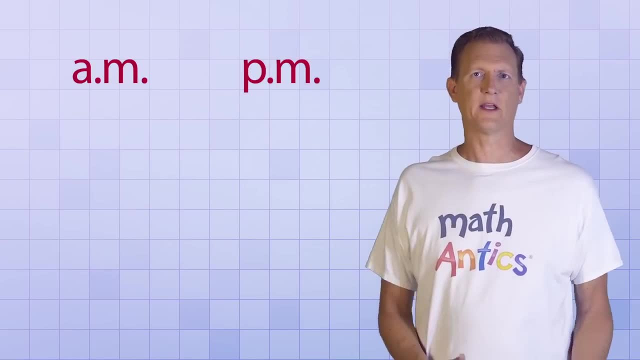 AM stands for anti-meridian, which just means before noon, And PM stands for post-meridian, which just means after noon. To see how the AM and PM labels work with the 12 hours on our clock face to keep track of a full day. 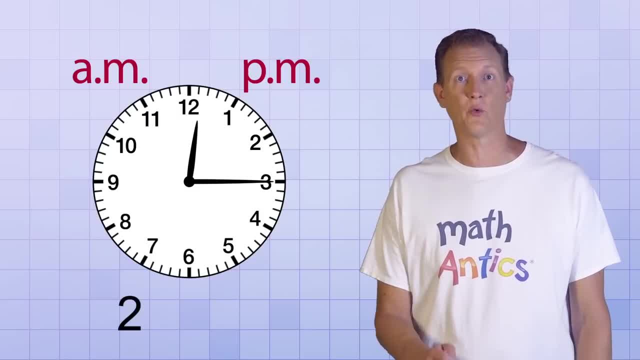 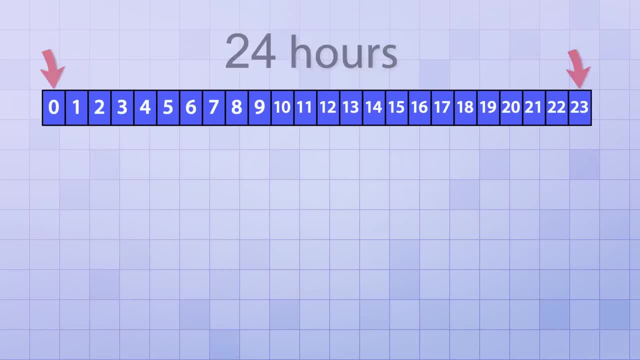 let's compare them to a simpler modern timekeeping system called the 24 hour clock. In that system, the 24 hours of the day are just labeled 0 through 23.. In other words, at the beginning of the day, which happens to be midnight, the time is 0 hours and 0 minutes. 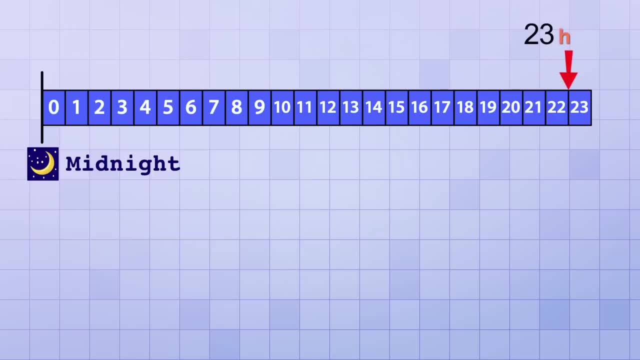 As the hours pass by, you eventually get to the time 23 hours and 0 minutes, which means you're starting the 24th hour of the day. After that last hour passes, it starts back over at 0 for the next day. 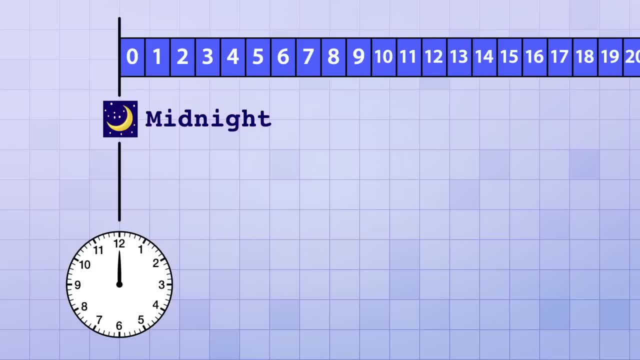 On the traditional clock face, at midnight, the hour hand is pointing straight up at 12.. So instead of calling it 0 o'clock, we call it 12 midnight or 12 AM. Then the first 12 hours of the day pass 1 minute and then the hour hand is pointing straight up at 12.. 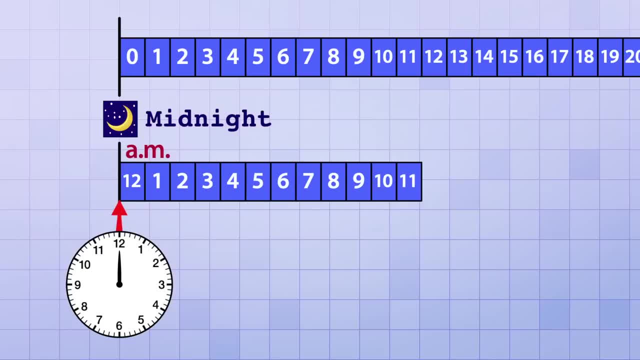 Then the first 12 hours of the day pass 1 minute and then the hour hand is pointing straight up at 12.. The hour hands now pass 1 by 1 using the AM label: 1 AM, 2 AM, 3 AM on up to 11 AM. 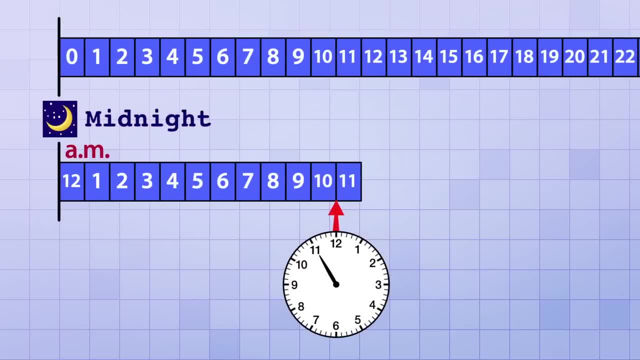 When the hour hand gets to 11 AM, you're beginning the 12th hour of the day, And as soon as the 60 minutes of that hour pass by, the hour hand will be back up at the top of the clock, pointing at 12 again. 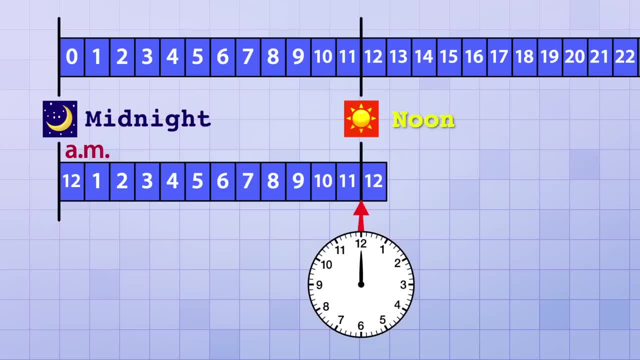 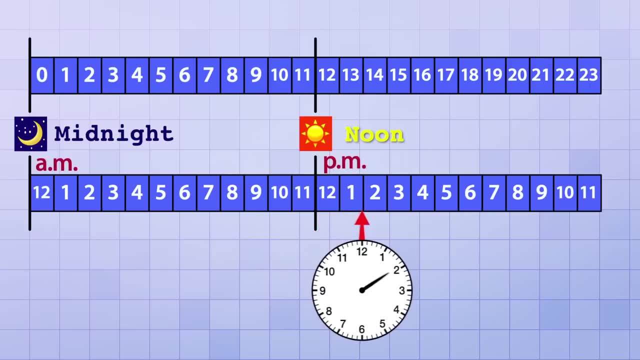 But this time we're gonna call that position 12 noon or 12pm. Then the clock continues counting out the last 12 hours of the day using the PM label: 1 PM, 2 pm, 3 pm on up to 11 pm. 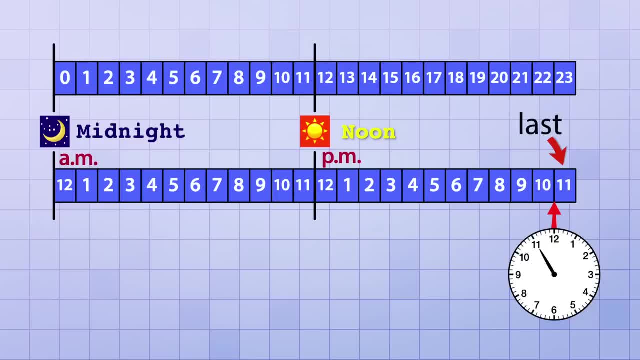 When the hour hand gets to 11 pm, it means you're starting the last or 24th hour of the day. After that last hour passes, the hour hand points straight up at 12 again, which is now 12 midnight or 12 am, and the cycle starts all over for the next day. 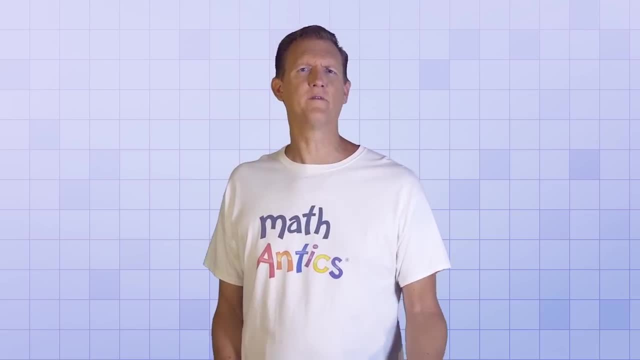 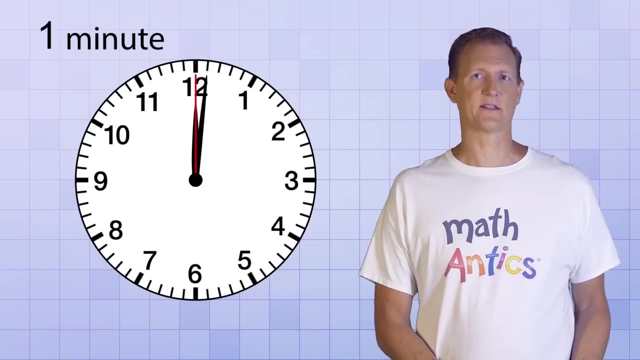 Let's briefly summarize what we've learned about the clock so far before moving on to a few examples of telling time. Each time the second hand rotates all the way around the clock, 1 minute has passed and the minute hand advances 1 mark. 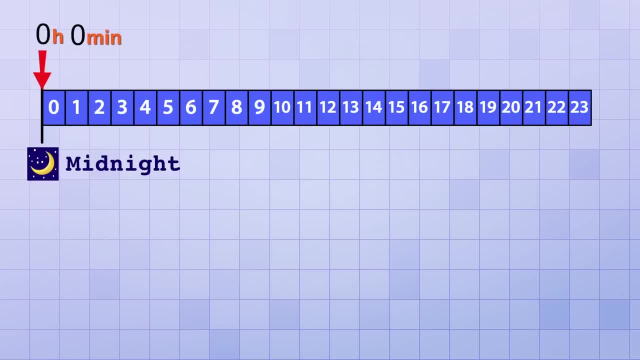 the time is… 0 hours and 0 minutes. As the hours pass by, you eventually get to the time 23 hours and 0 minutes, which means you're starting the 24th hour of the day. After that last hour passes, it starts back over at 0 for the next day. 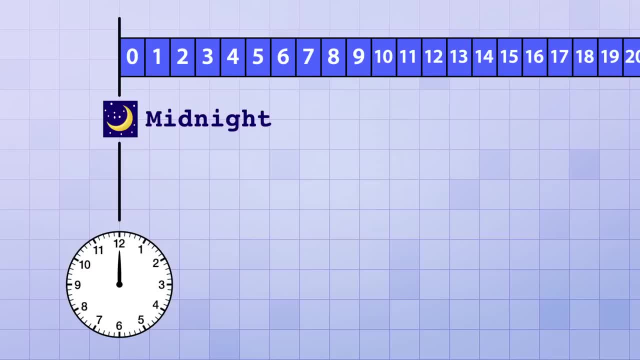 On the traditional clock face at midnight, the hour hand is pointing straight up at 12.. So instead of calling it 0 o'clock, we call it 12 midnight or 12 AM. Then the first 12 hours of the day pass one by one using the AM label. 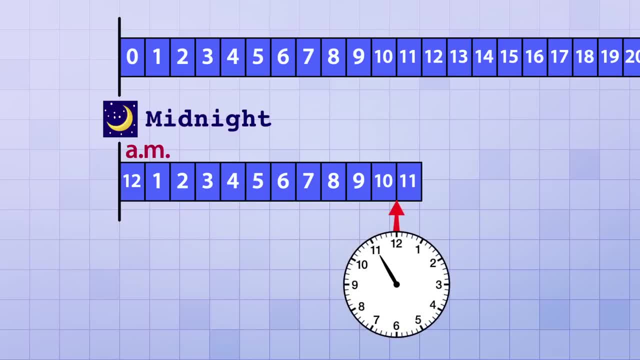 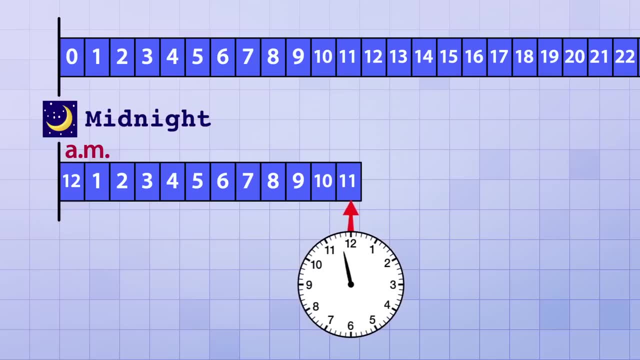 1 AM, 2 AM, 3 AM on, up to 11 AM. When the hour hand gets to 11 AM, you're beginning the 12th hour of the day, And as soon as the 60 minutes of that hour pass by. 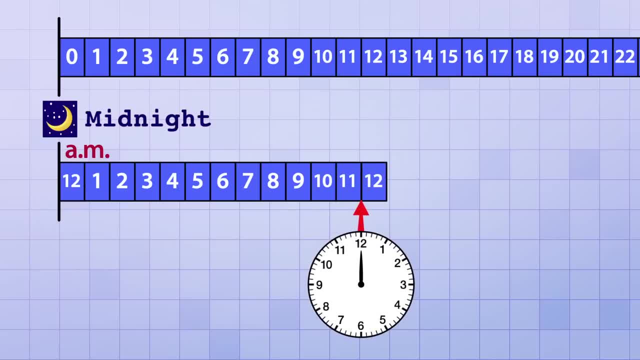 the hour hand will be back up at the top of the clock, pointing at 12 again, But this time we're going to call that position 12 noon or 12 PM. Then the clock continues on counting out the last 12 hours of the day using the PM label. 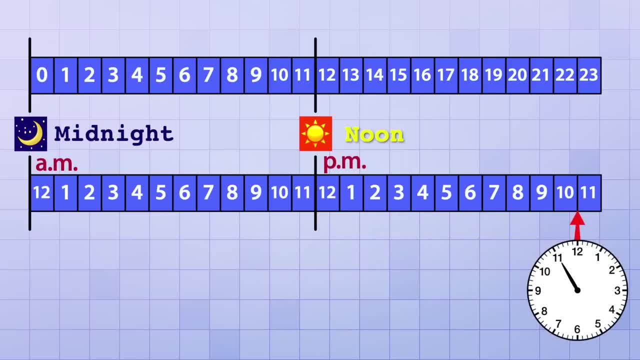 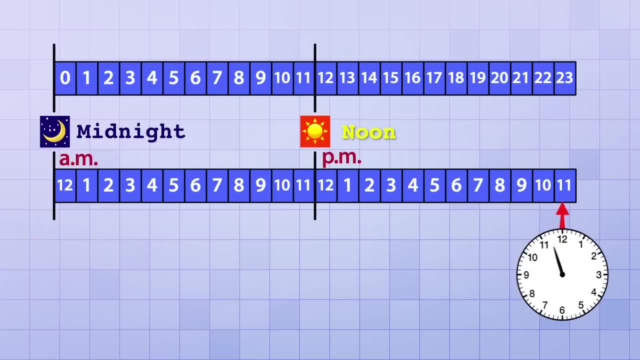 1 PM, 2 PM, 3 PM on up to 11 PM. When the hour hand gets to 11 PM, it means you're starting the last or 24th hour of the day. After that last hour passes, the hour hand points straight up at 12 again. 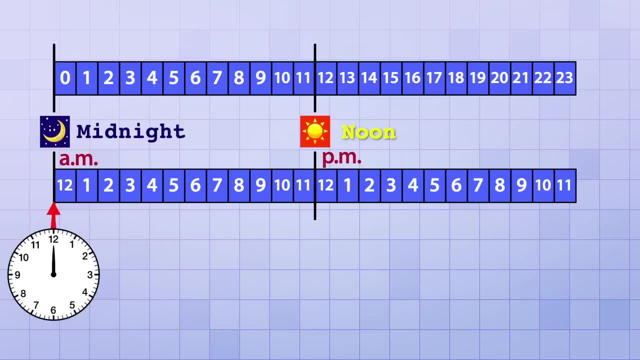 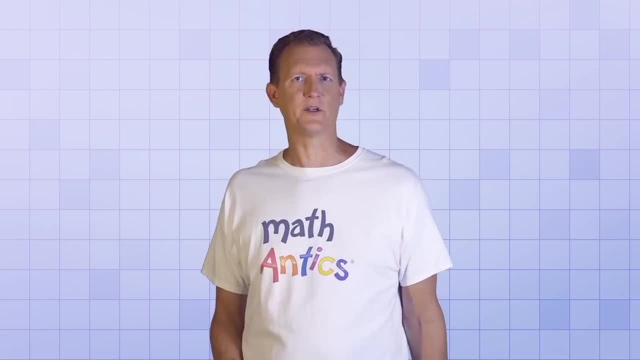 which is now 12 midnight or 12 AM, And the cycle starts all over for the next day. Let's briefly summarize what we've learned about the clock so far, before moving on to a few examples of telling time. Each time, the second hand rotates all the way around the clock. 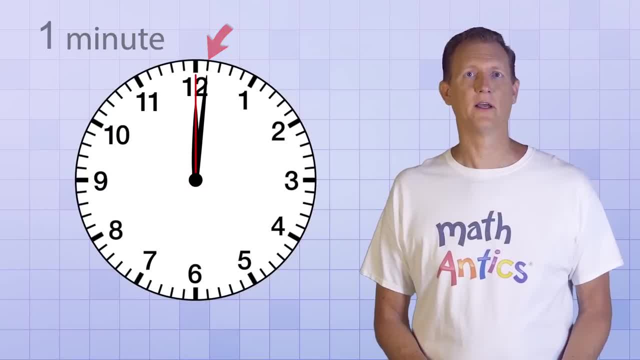 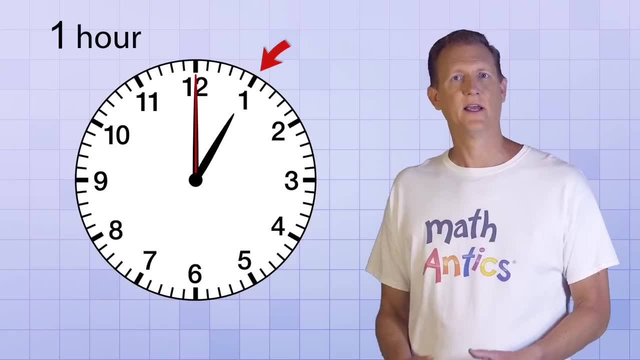 one minute has passed and the minute hand advances one mark Each time the minute hand goes all the way around the clock. one hour has passed and the hour hand advances 5 marks Each time the hour hand goes around the clock. 12 hours have passed, which is half a day. 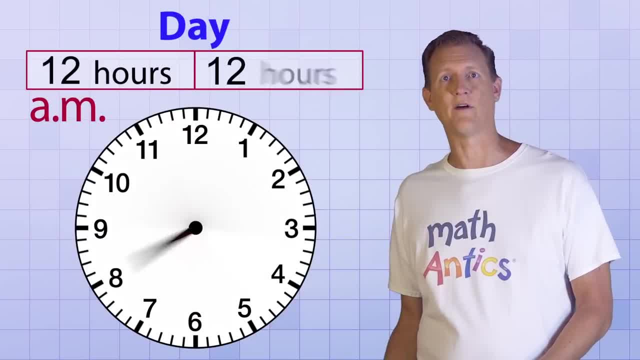 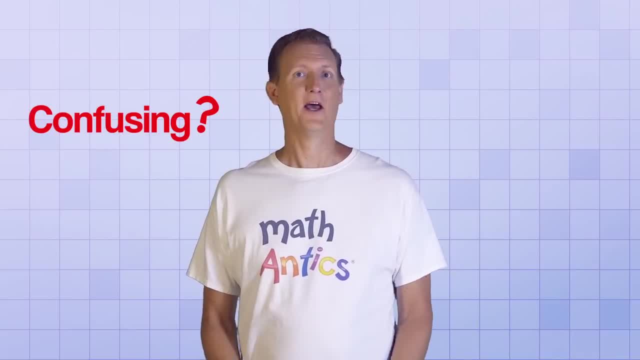 The first 12 hours are called the AM hours and the second 12 hours are called the PM hours. If this is your first time learning how a clock works, it might seem kind of confusing. But don't worry, The more you practice looking at a clock and noticing which hands are pointing to which marks, 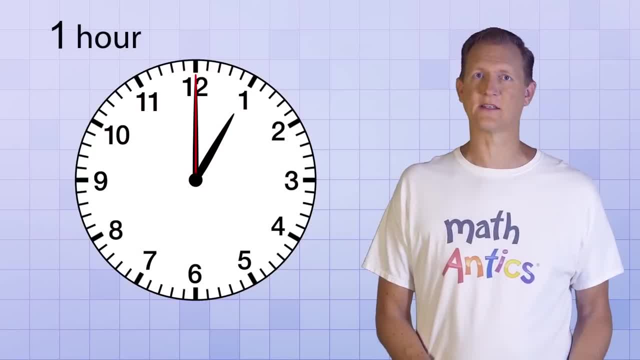 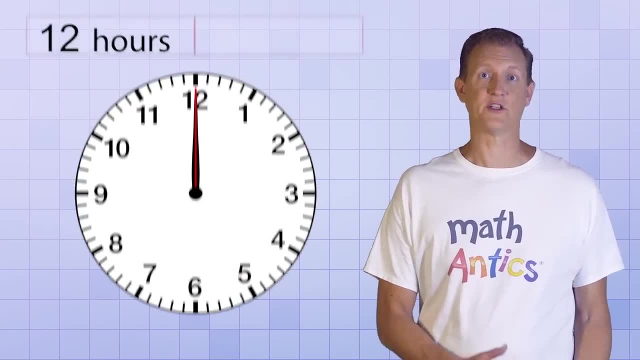 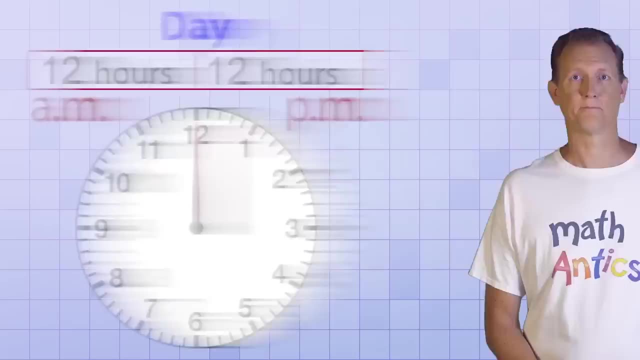 Each time the minute hand goes all the way around the clock, 1 hour has passed and the hour hand advances 5 marks. Each time the hour hand goes around the clock, 12 hours have passed, which is half a day. The first 12 hours are called the am hours and the second 12 hours are called the pm hours. 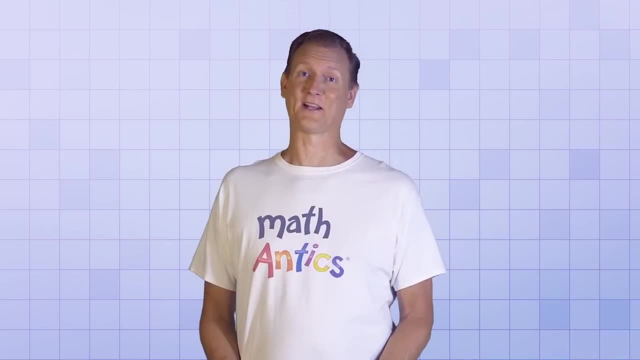 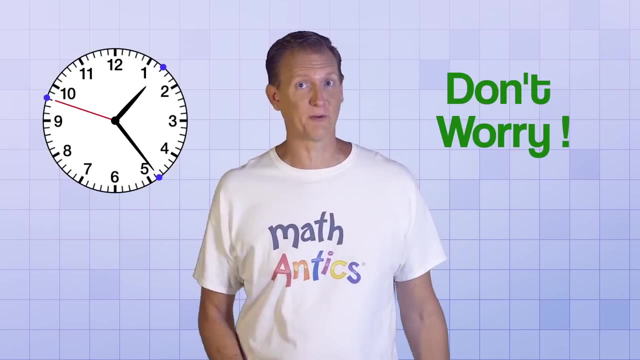 If this is your first time learning how a clock works, it might seem kind of confusing, But don't worry. The more you practice looking at a clock and noticing which hands are pointing to which marks, the faster you'll be able to tell what time it is. 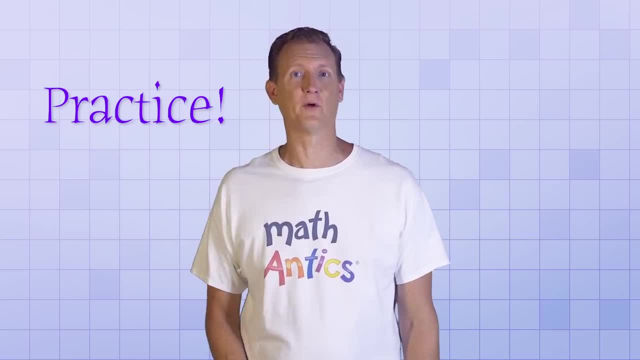 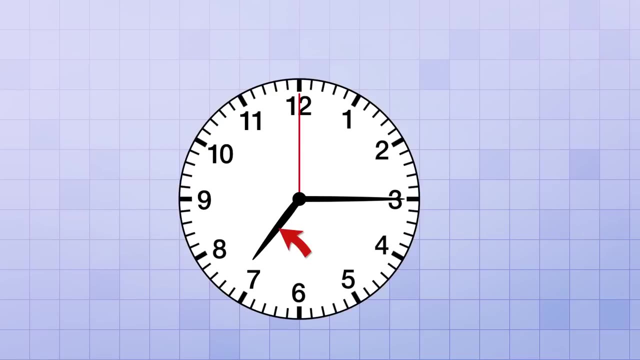 In fact, let's practice that a few times now so you can get the hang of it, before doing more practice on your own. Let's start with this clock face. What time of day is it displaying? The hour hand is past the 7, but not to 8 yet, so the hour is 7.. 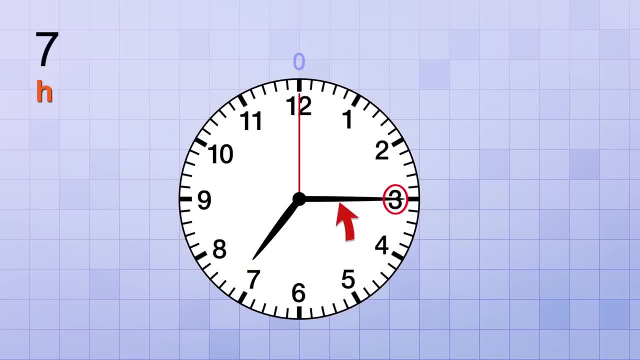 The minute hand is pointing directly at the 3, but remember that's the third group of 5 marks for counting minutes or seconds. So it's pointing… the 15 minute mark. And the second hand is pointing straight up, which is the 0 second mark. 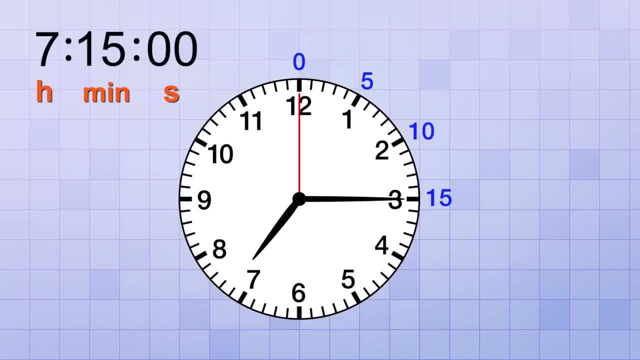 So the time is 7 hours 15 minutes and 0 seconds. Oh, and that's how you write time using numbers. You write the hours first, then minutes and then seconds, if necessary, all separated by colons. But is this 7.15 am or pm? 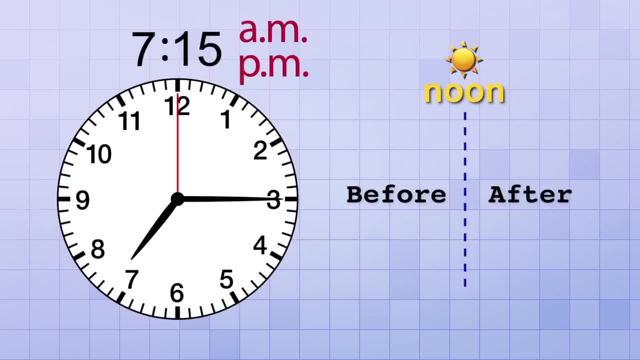 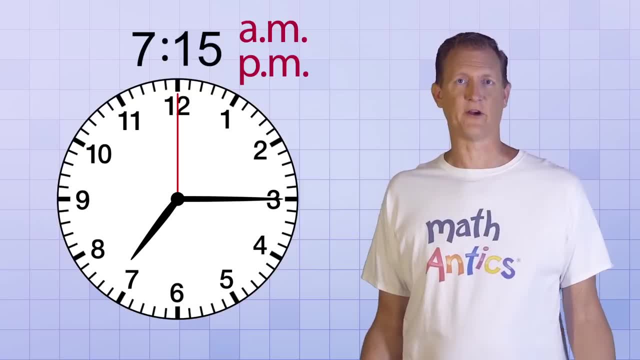 To tell that you need to know if it's before noon or afternoon, the halfway point of the day. Books or tests sometimes give you a clue about whether the time is before noon or afternoon, So you can figure it out, Or they may just tell you if it's am or pm. 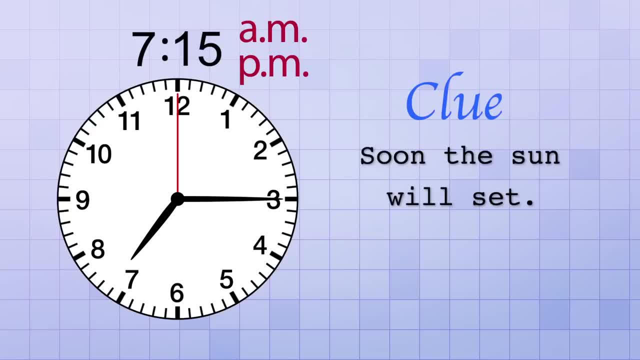 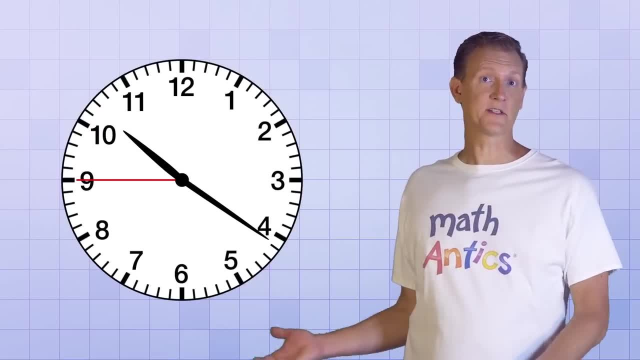 In this case we're given the clue: Soon the sun will set, so we know it's afternoon or 7.15 pm. How about this example? What time is this clock displaying? The hour hand is past the 10,, but not to 11 yet, so the hour is 10.. 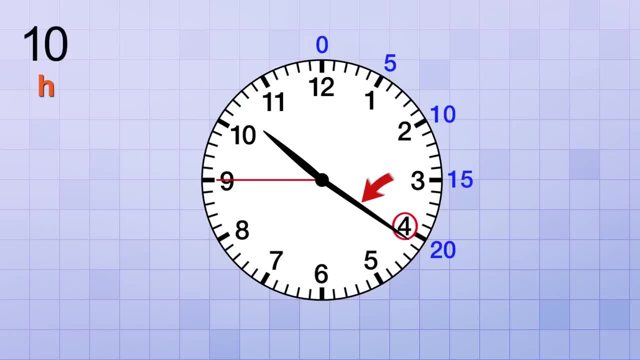 The minute hand is just past the 4,, which is the 20 minute mark, but it's not to 21 yet, so the minute is 20.. And the second hand is past the 4,, which is the 4 seconds. 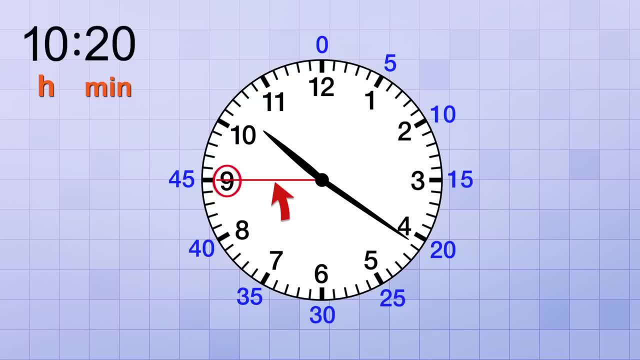 Which means is pointing at the 9,, which is the 45 second mark. So the time is 10 hours 20 minutes and 45 seconds, And this time you're given the clue: it's a beautiful morning, so you know that it's. 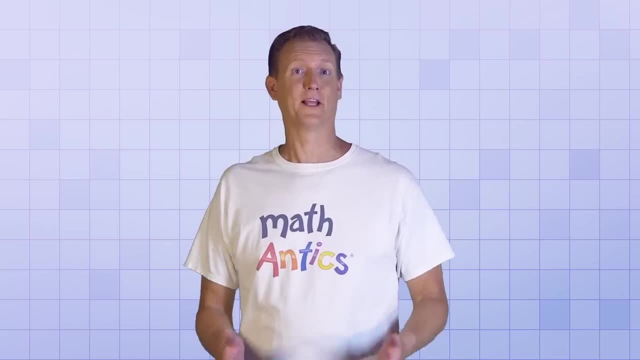 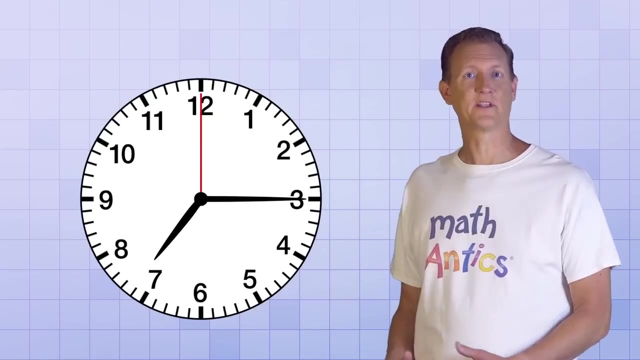 the faster you'll be able to tell what time it is In fact. let's practice that a few times now so you can get the hang of it before doing more practice on your own. Let's start with this clock face. What time of day is it displaying? 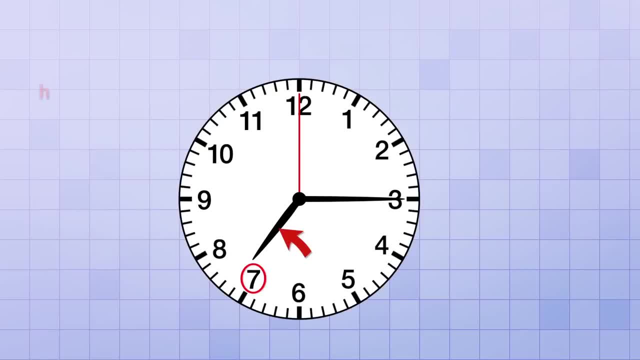 The hour hand is past the 7, but not to 8 yet, so the hour is 7.. The minute hand is pointing directly at the 3,, but remember that's the third group of 5 marks for counting minutes or seconds. 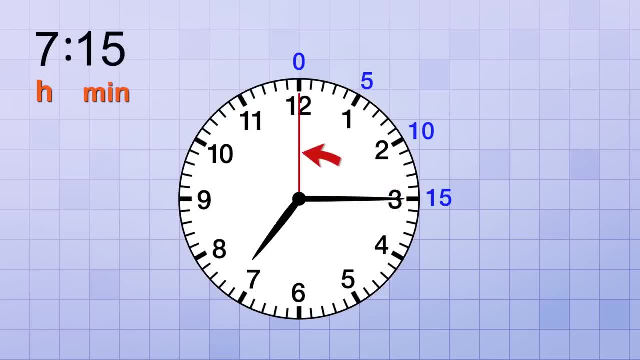 So it's pointing at the 15 minute mark And the second hand is pointing straight up, which is the 0 second mark. So the time is 7 hours 15 minutes And 0 seconds. Oh, and that's how you write time using numbers. 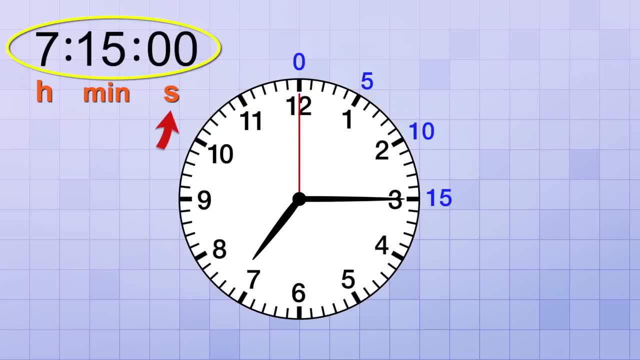 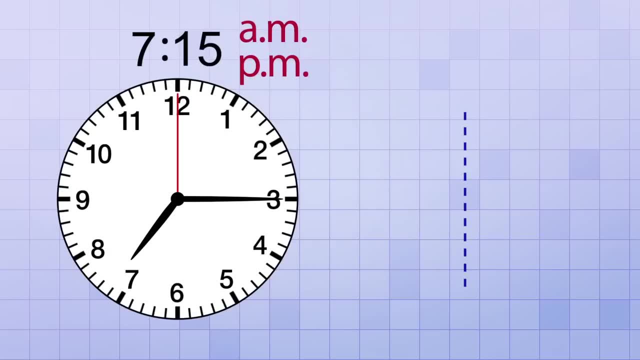 You write the hours first, then minutes and then seconds, if necessary, all separated by colons. But is this 7.15 am or pm? To tell that you need to know if it's before noon or afternoon, the halfway point of the day. 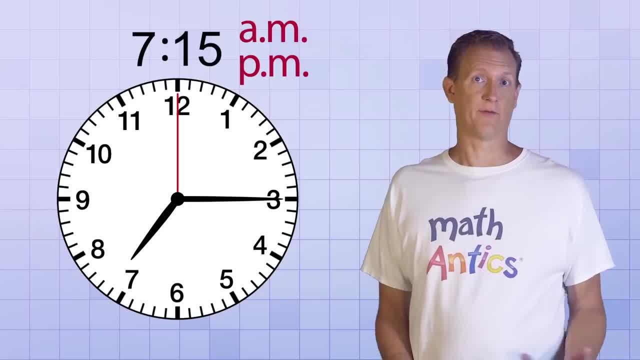 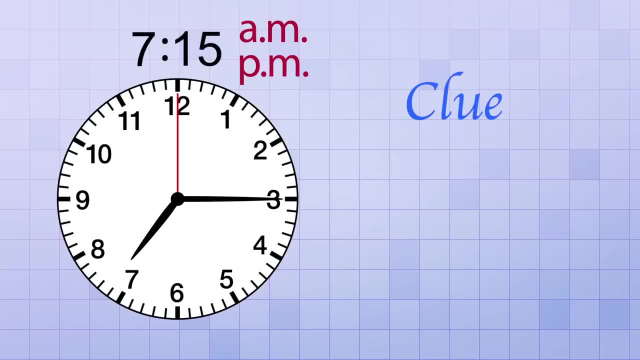 Books or tests sometimes give you a clue about whether the time is before noon or afternoon, so you can figure it out, Or they may just tell you if it's am or pm. In this case, we're given the clue…. 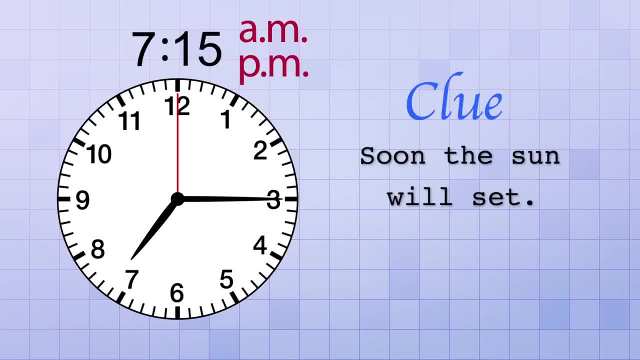 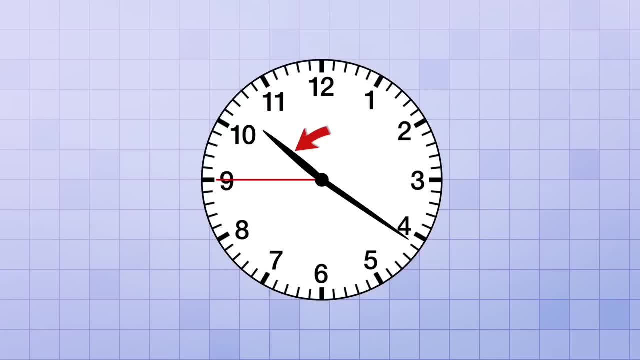 Soon the sun will set. So we know it's afternoon or 7.15 pm. How about this example? What time is this clock displaying? The hour hand is past the 10, but not to 11 yet, so the hour is 10.. 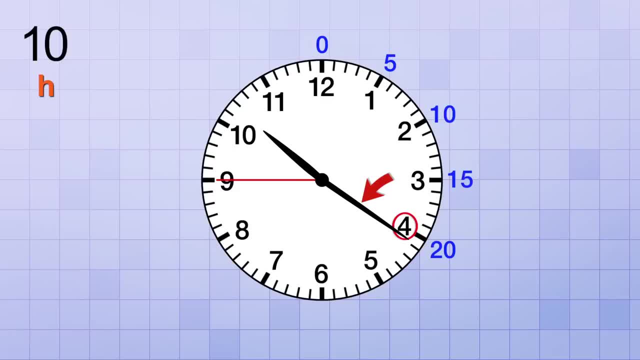 The minute hand is just past the 4,, which is the 20 minute mark, but it's not to 21 yet, so the minute is 20.. And the second hand is pointing at the 9,, which is the 45 second mark. 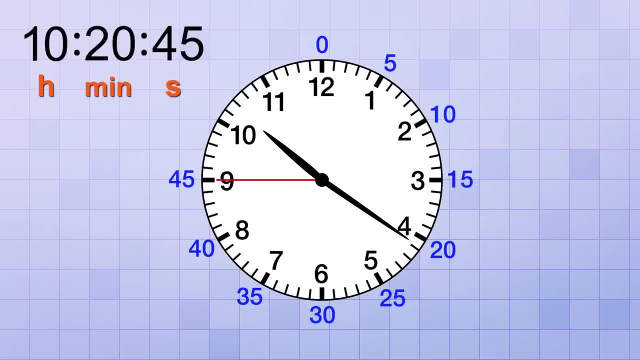 So the time is 10 hours 20 minutes and 45 seconds. This time you're given the clue…. It's a beautiful morning. so you know that it's 10.20 am, since morning comes before noon. 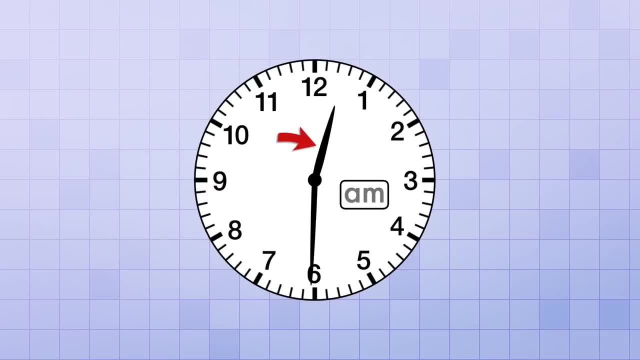 And finally… What time of day is this clock displaying? The hour hand is past the 12,, but not yet to the 1,, so it's 12 something. The minute hand is pointing just a hair past the 6,, which is the 30 minute mark. 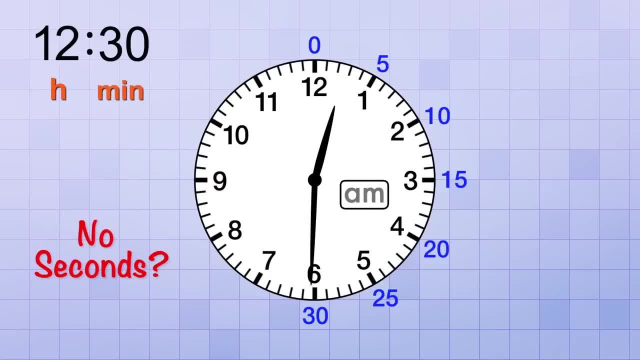 so the minute is 30.. And there's no second hand on this clock. Not all clocks have them, So we're only concerned about the time to the nearest minute in this example. Lastly… this clock face is actually labeled AM, so we know that the time of day is 1230 AM.